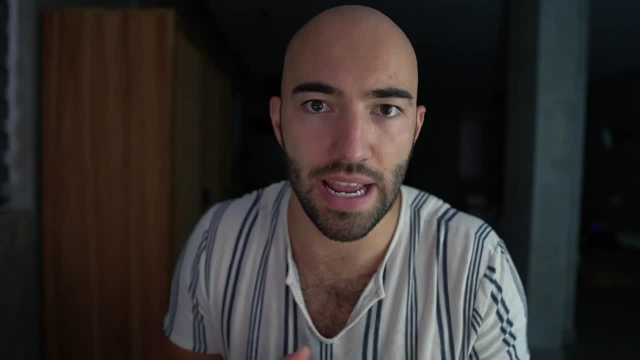 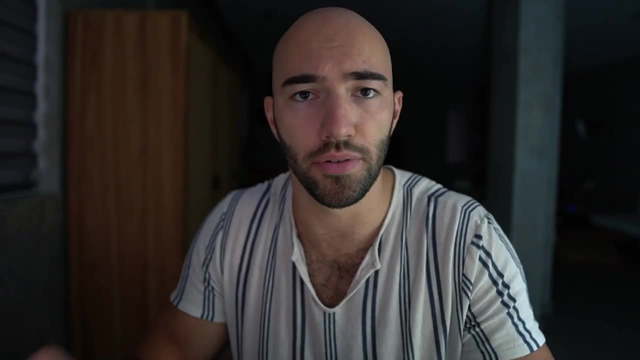 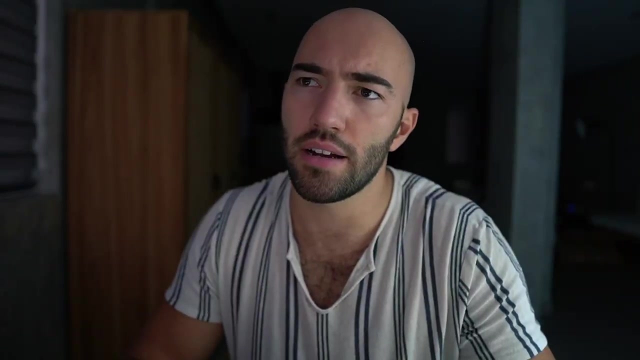 models. Those are models that understand different domains of information, like for clip, for example, that is, image and text. But how about other state-of-the-art computer vision models? How do they perform in comparison? Well, these other computer vision models, they are characterized by: 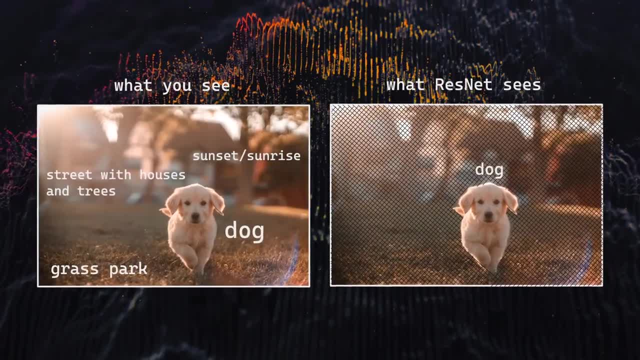 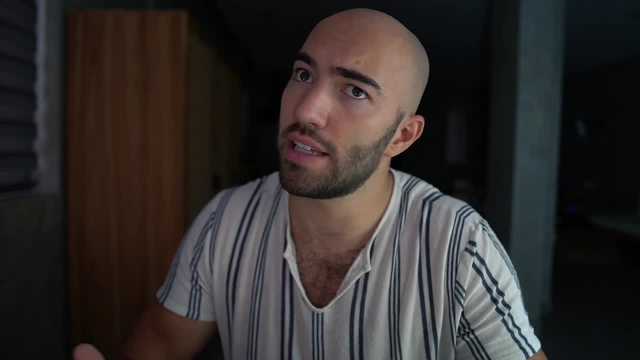 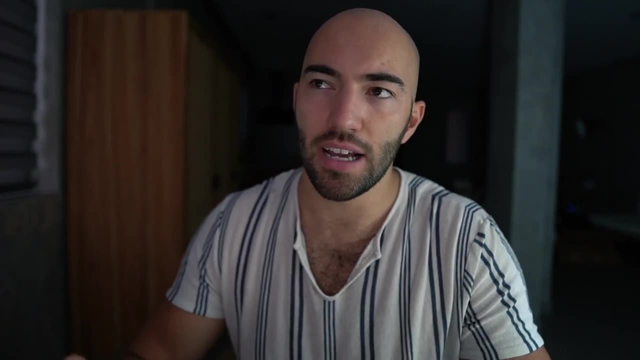 the fact that they really focus on one thing in an image. So, for example, let's say we had a computer vision model that was trained to classify an image as to whether it contained a dog, a car or a bird. A computer vision model doesn't really need to know anything other than what a car looks like. 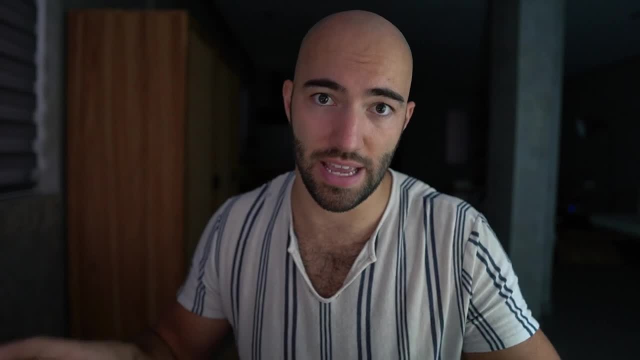 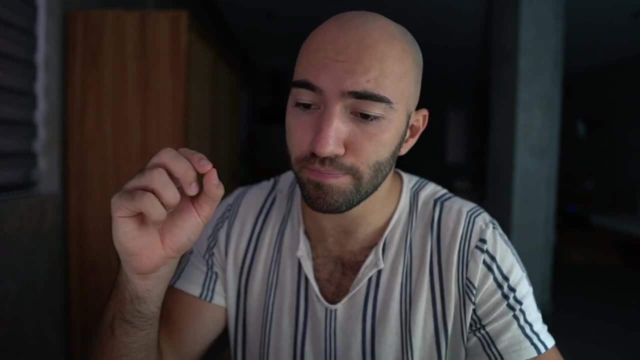 what a dog looks like and what a bird looks like. It can ignore everything else in those images, and that's one of the limitations of the state-of-the-art computer vision models. They have been pre-trained on a huge amount of data, but they've been pre-trained for 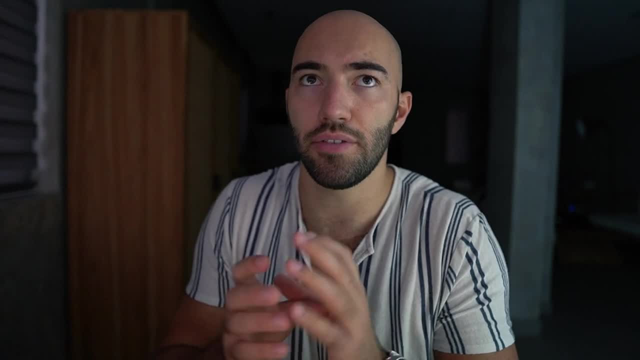 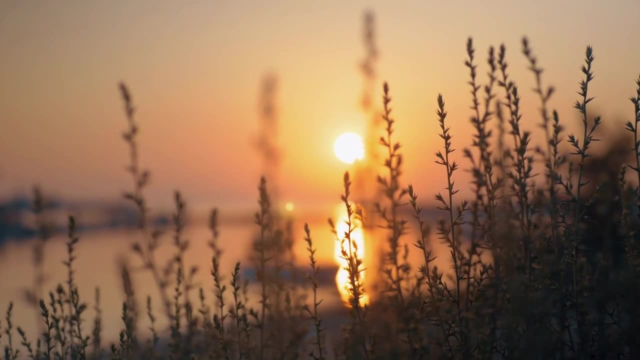 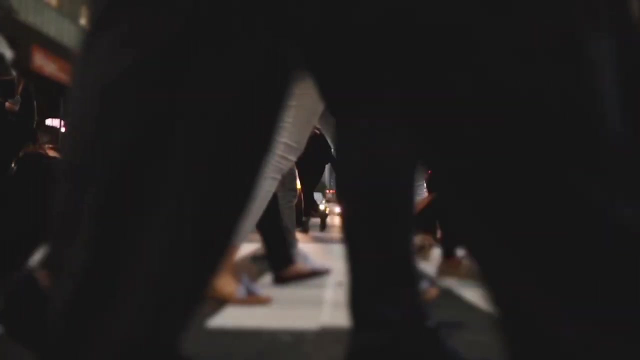 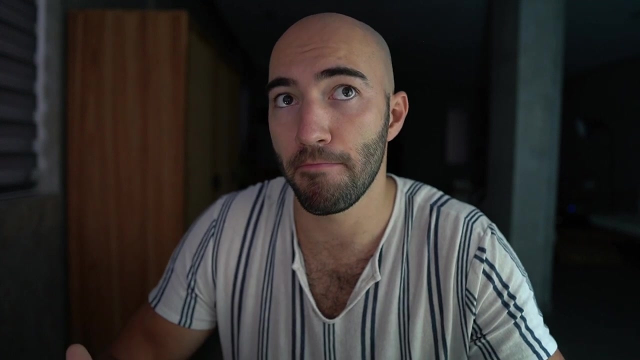 classification of these particular elements, and even if you have like a thousand or ten thousand classes in there, that hardly represents the real world, which has a huge variety of concepts and objects for us to, as humans, to to understand and see and categorize. So what we find with these computer vision models is that they perform. 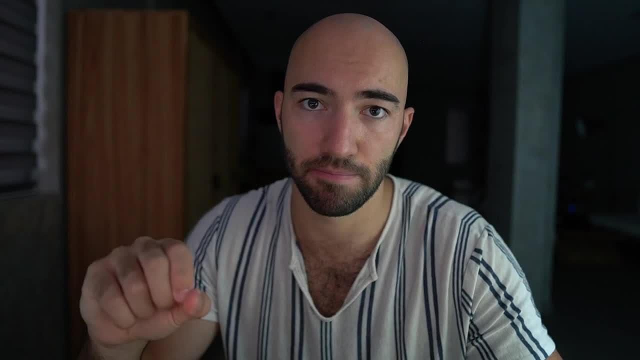 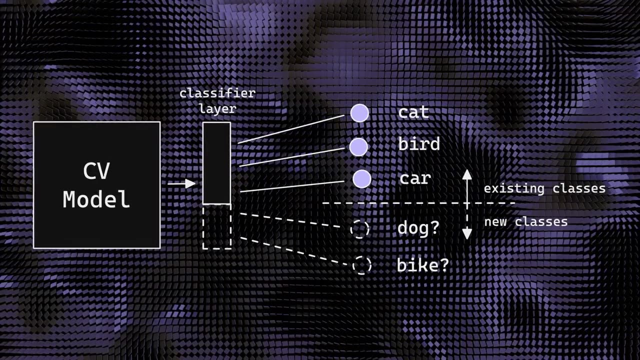 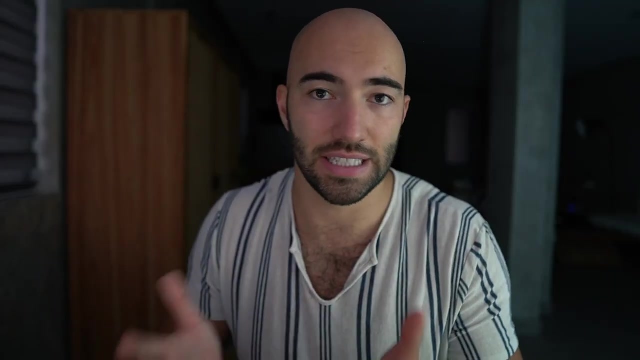 very well on specific data sets, but they're not so good at handling new classes. for example, For that model to understand a new class of objects and images will need to be fine-tuned further and it's going to need a lot of data and it's just, it's not very. 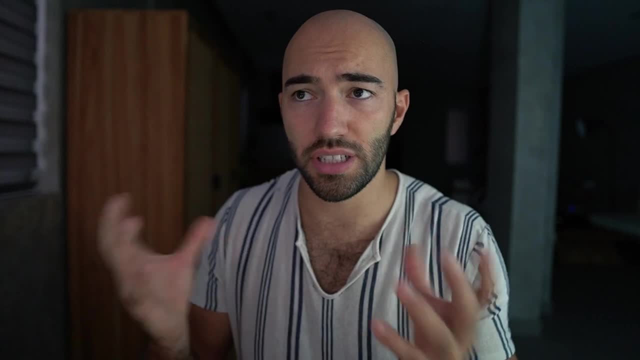 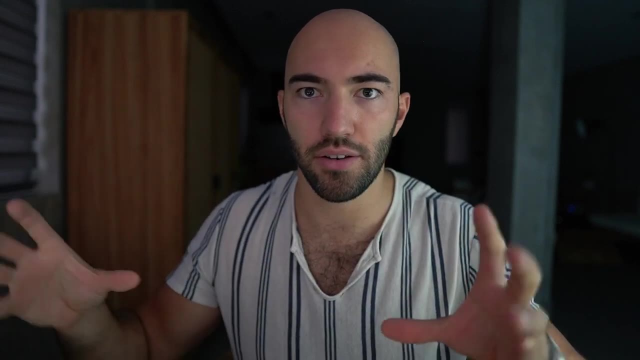 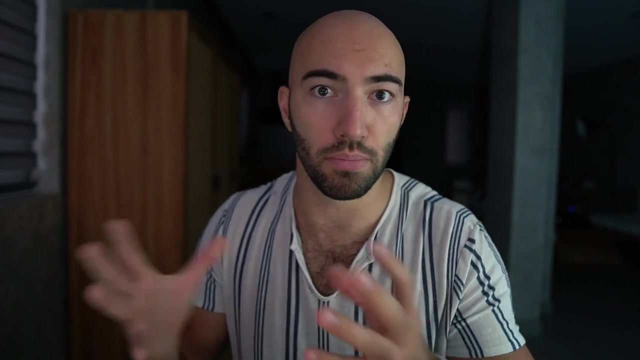 easy to do. Ideally we want a computer vision model to just understand kind of not everything would be perfect. obviously we're not quite there yet, but if it can just understand the world and the visual world relatively well, then we're sort of on the way to a more robust model. 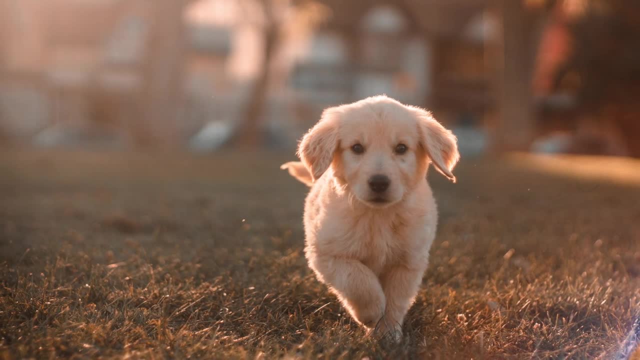 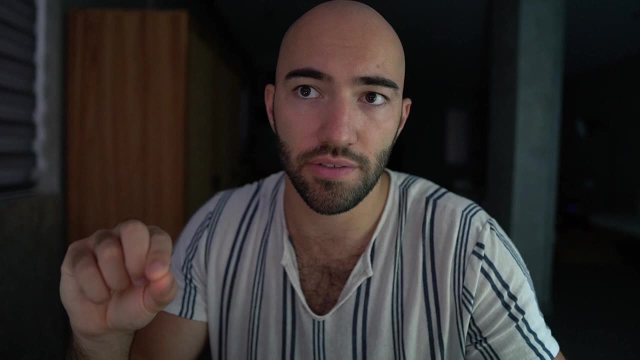 So, for example, this image of a dog, we want the model to understand that dog is in the image and you know, usually use convolutional neural network. that sort of model for image classification will know that there is a dog in the image but it doesn't. it doesn't care about everything else. 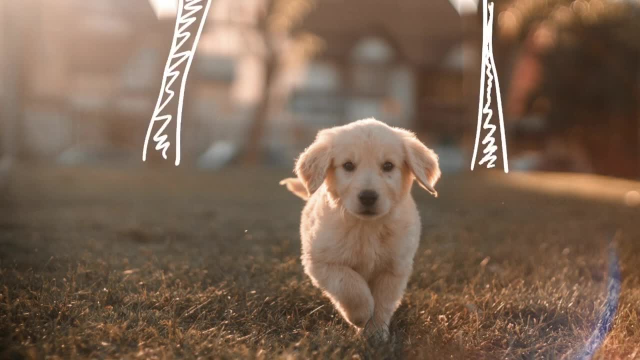 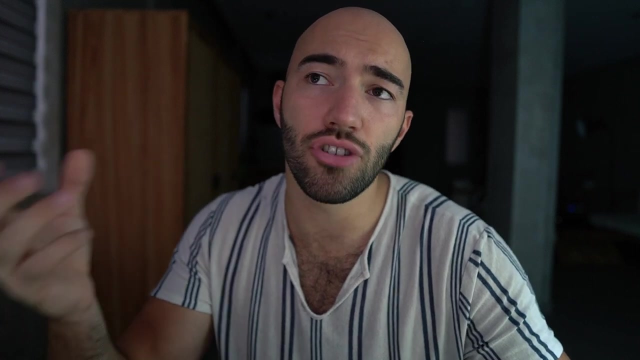 in the image. Ideally, we wanted to understand that there are trees in the background, the dog is running towards the camera, it's on aggressive field, it's sunrise or sunset, and that there are some blurry trees in the background- the blue street. Unfortunately, classification training- we don't get that. Instead, the models are essentially just learning to push their internal. 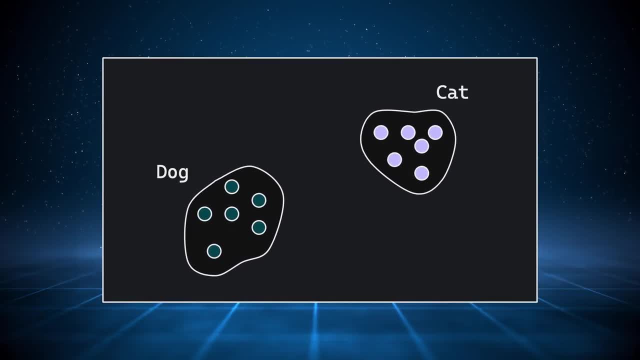 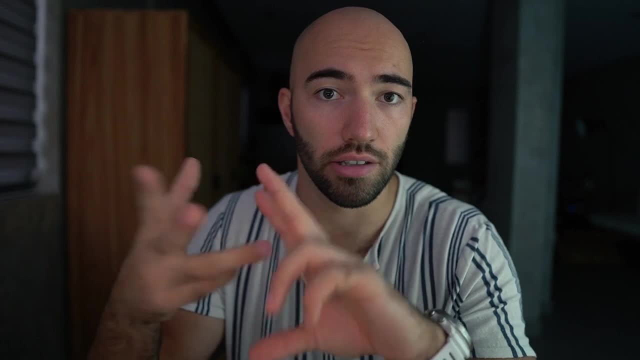 imaginations of images with dogs in all towards the same sort of vector space. That's essentially how we can, we can think about this and then, for example- earlier I said- cars and birds as well we could imagine. so they have like a cluster of dog images, they have a cluster of bird images and they 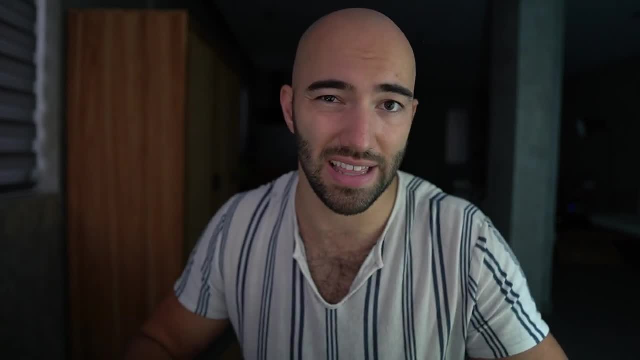 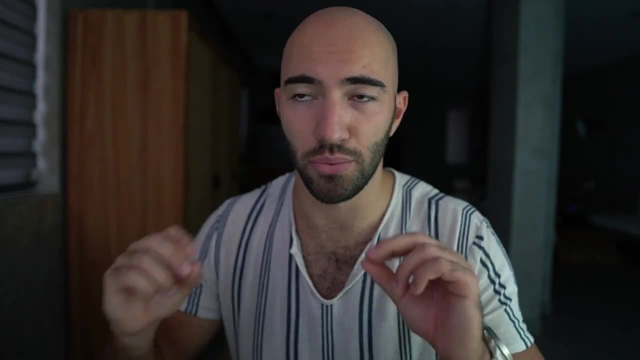 have a cluster of car images, but they don't really have anything else in between that. So this is ideal. if we just want a yes or no answer for a specific data set and we want good performance, we can do that as long as we have the training data and the computer. 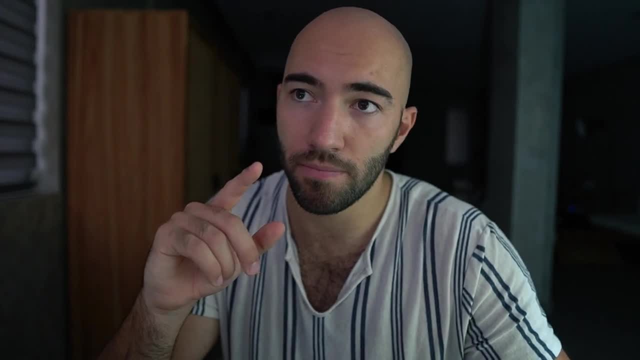 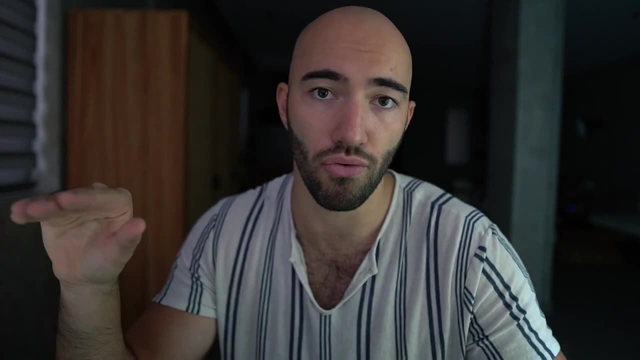 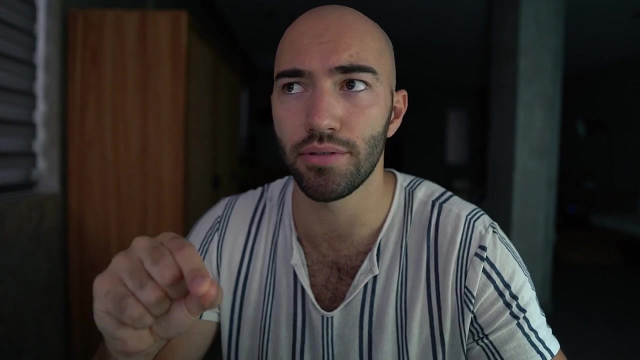 However, if we don't have all of that and we just want good performance- maybe not state-of-the-art, but good performance across a whole range of data sets- that's where we use CLIP. CLIP has proved itself as an incredibly flexible model that can work in both text and images, and 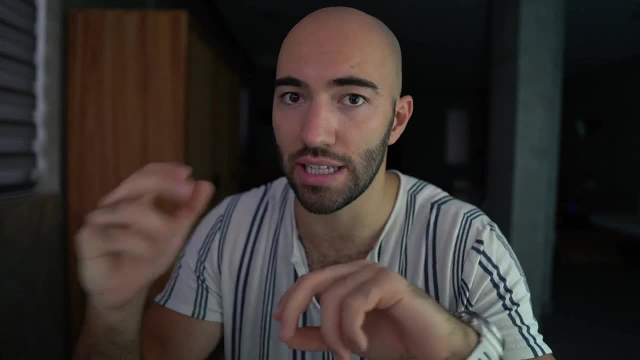 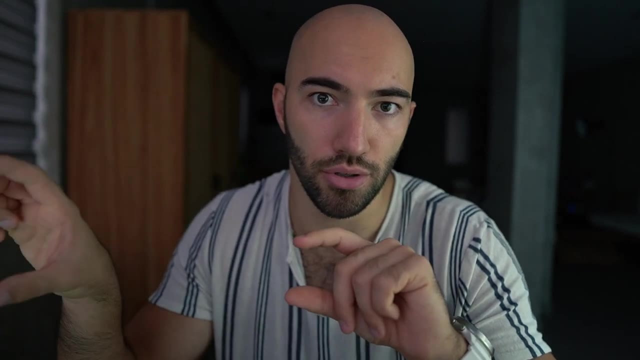 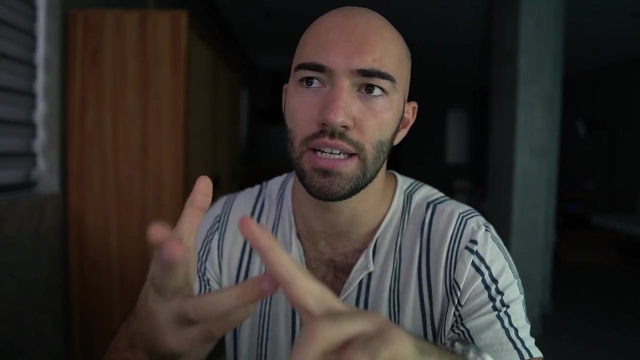 is amazing at what something we call zero-shot classification. Zero-shot basically saying you need zero training examples for this model to adapt to a new domain. So before we dive into CLIP, let's just explain this zero-shot thing in a little more detail. So zero-shot comes from? 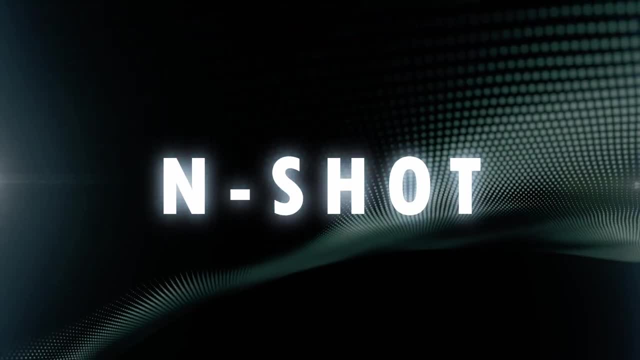 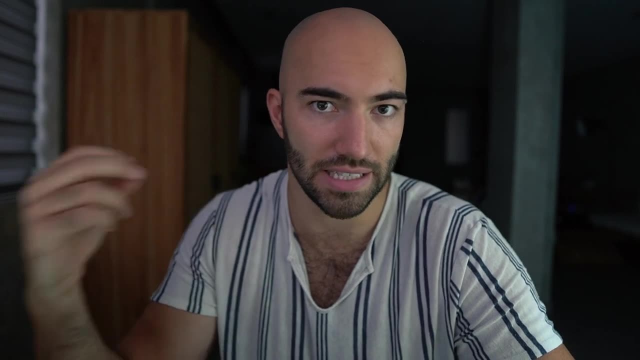 something called end-shot learning. End-shot, you may have guessed, is basically the number of training examples that you need for your model to perform on a particular new domain or new data set. Many state-of-the-art image classification models they tend to be pre-trained on, like ImageNet. 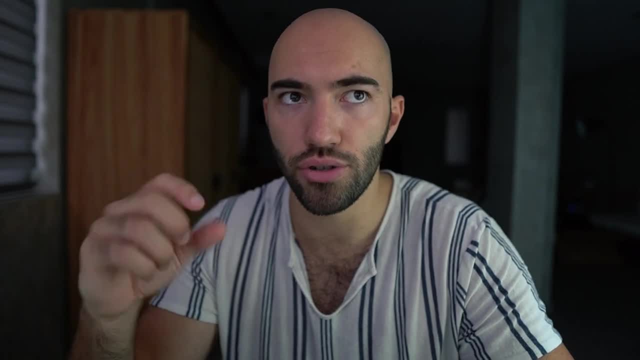 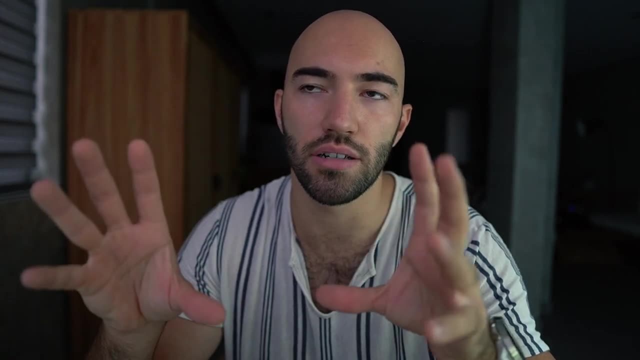 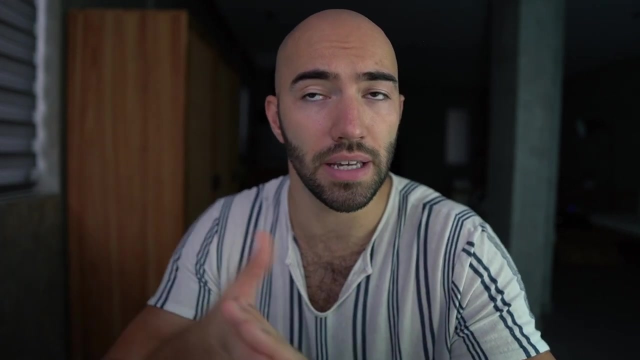 and then they're fine-tuned for a specific task. So they have the pre-training and the pre-training basically sets up the internal model weights of that model to understand the visual world, at least within the scope of the ImageNet classification set, which is fairly big. 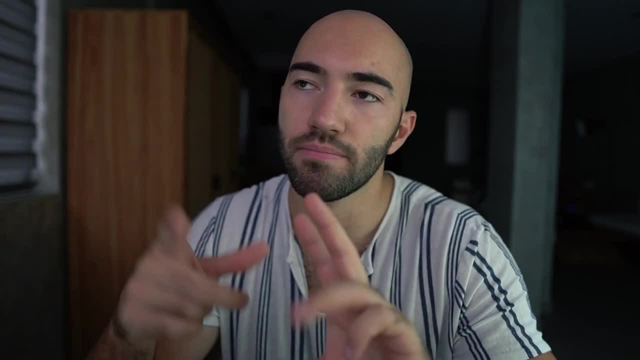 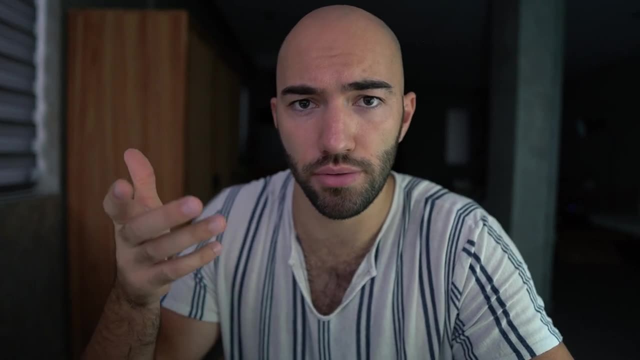 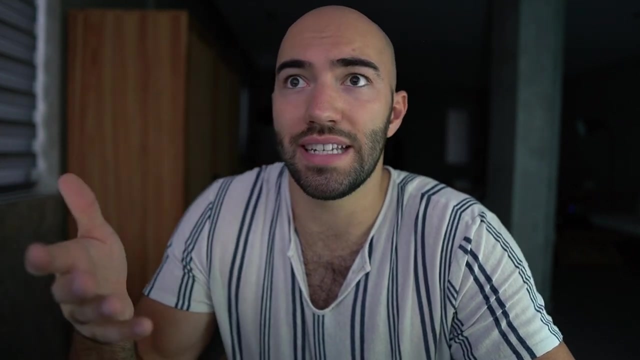 but it's obviously not as big as the actual world. And then those models are usually fine-tuned on a particular data set. and to fine-tune that pre-trained image classification model on a new domain you are going to need a lot of examples. 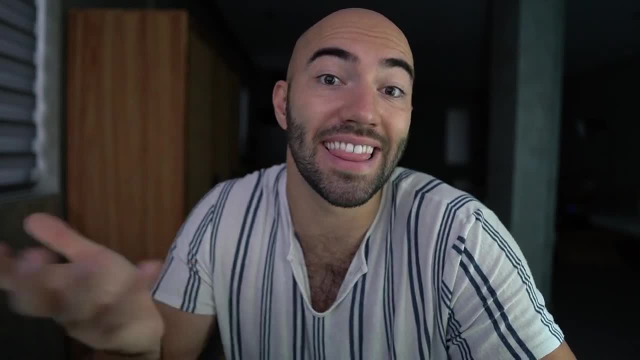 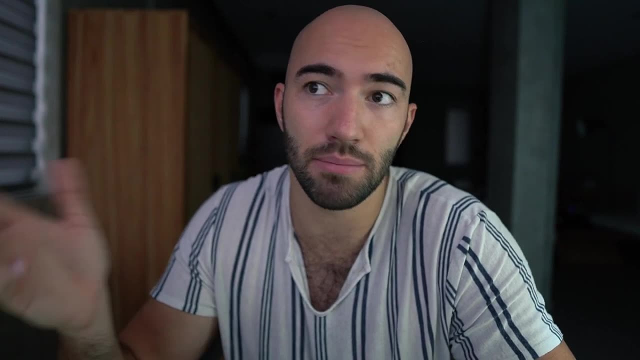 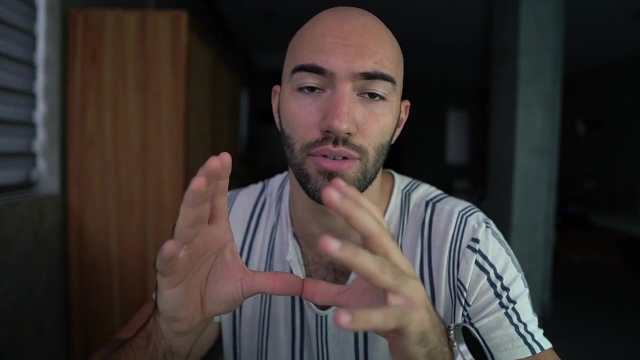 Let's say, as a rule of thumb, maybe you need 10,000 images for each class or each label within your data set. That may be excessive, it may be too little, I'm not sure, but you do need something within that ballpark in order to get good performance. We could refer to some of the 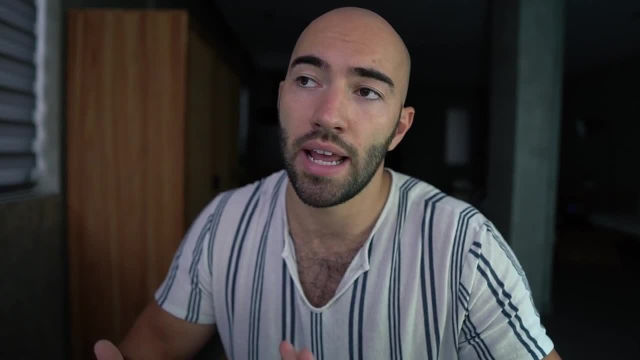 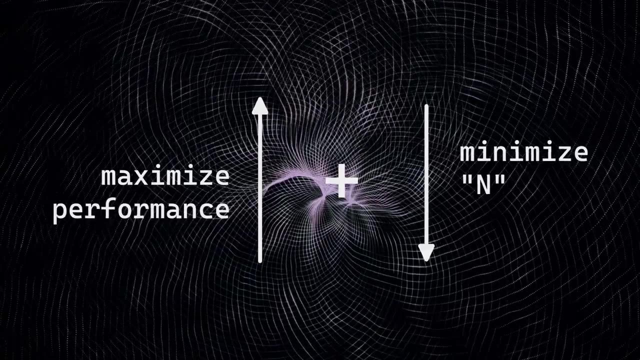 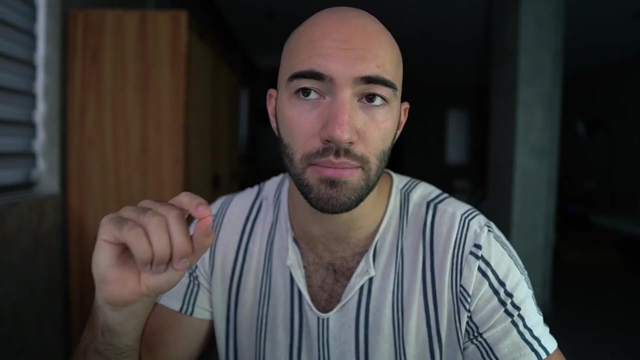 models. so these are like ResNet and BERT: as many shot learners. They need many, many training examples in order to learn a new domain. Ideally, we want to maximize model performance whilst minimizing the n in n shots. Okay, so minimizing the number of training examples needed for the 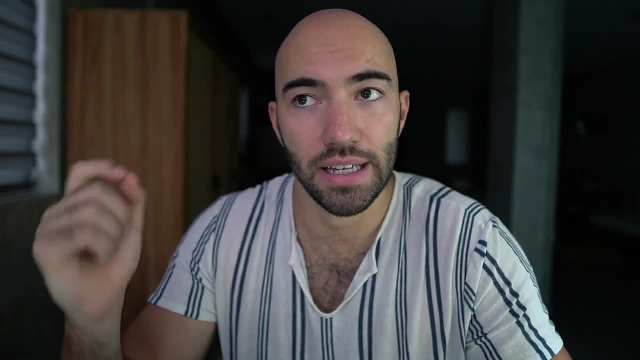 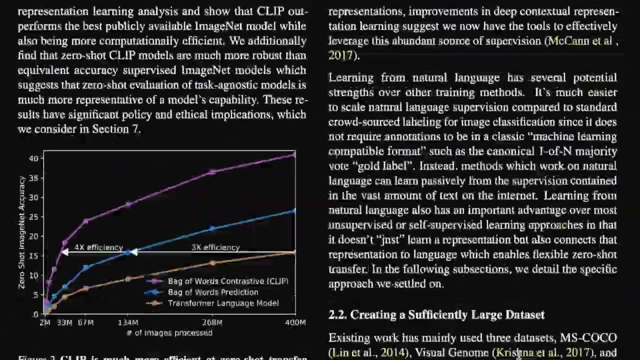 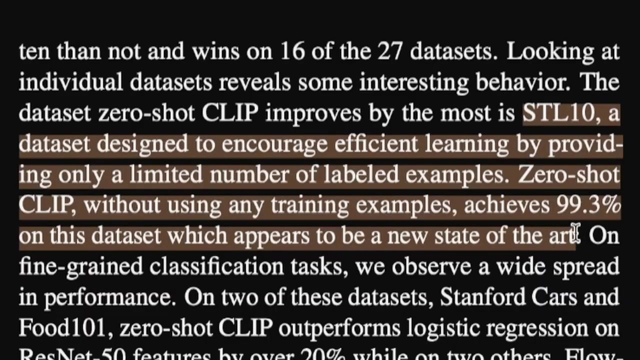 model to perform well Now. so I was noting that CLIP is not achieving state-of-the-art performance on any particular data sets or benchmarks Other than one. surprisingly, without seeing any training data for this particular data set, CLIP did actually get state-of-the-art performance on that one data set, which is surprising. 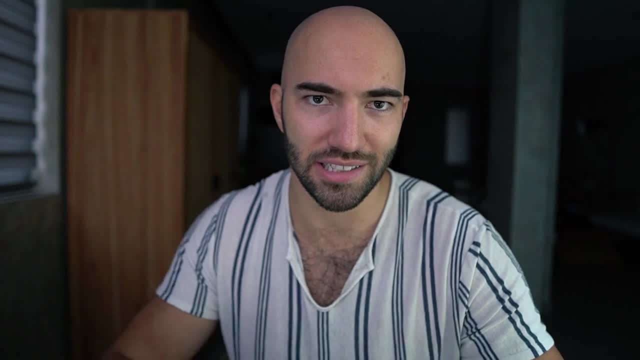 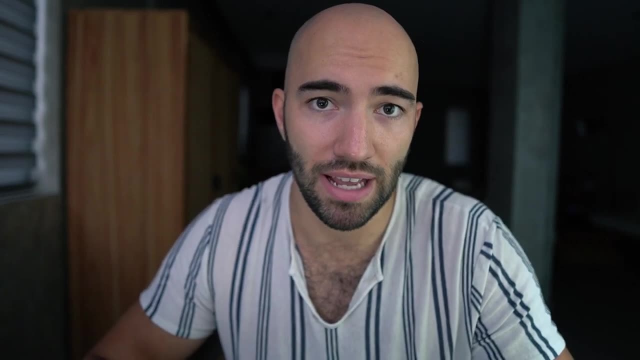 without seeing any of the training data. but here we go. this is. this is how useful this sort of thing is. Let's talk about how CLIP makes zero-shot learning so effective. So CLIP stands for contrastive language image pre-training. It was released by OpenAI in 2021.. 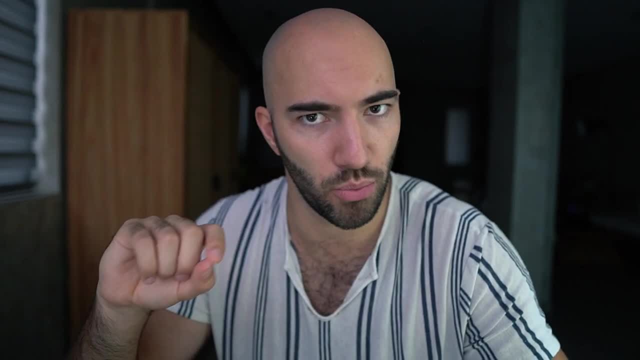 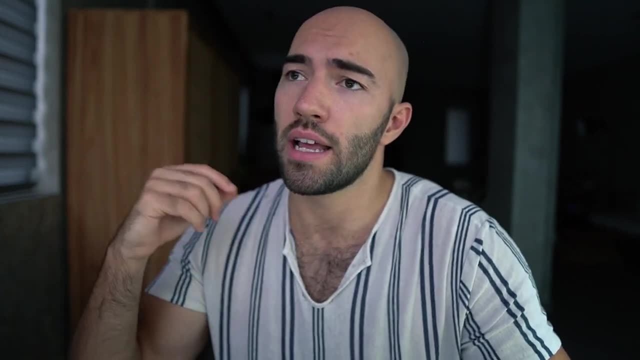 Since then it has done pretty well. We can find it in a lot of different use cases. this is just one of them. So CLIP itself actually consists of two models. I've discussed this in a previous video and article in a lot more detail. so if you're interested, go and. 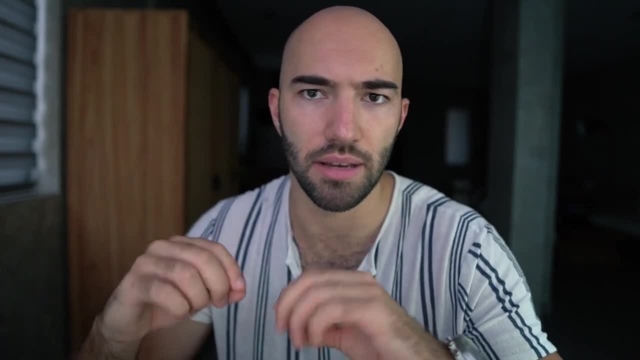 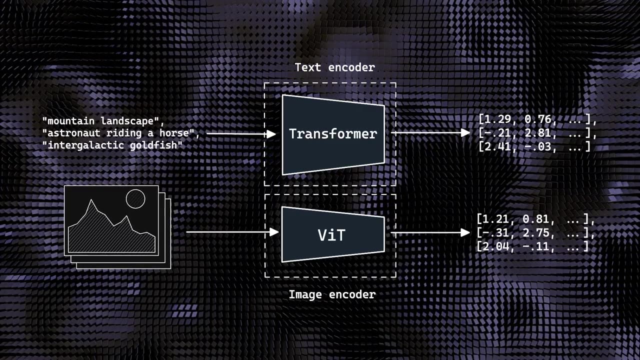 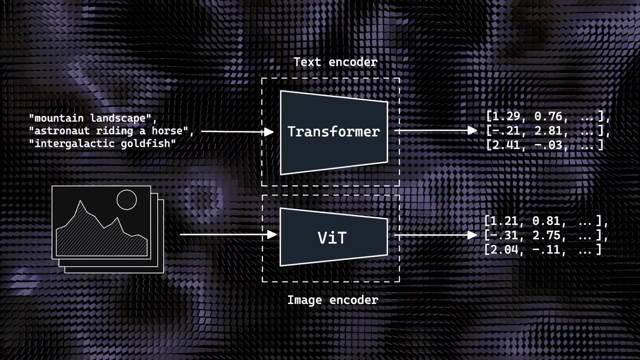 and have a look at that. For now we're going to keep things pretty light on how CLIP works. But in this version of CLIP those two models are going to consist of a typical text transformer model for dealing with the text encoding and a vision transform model for dealing with the 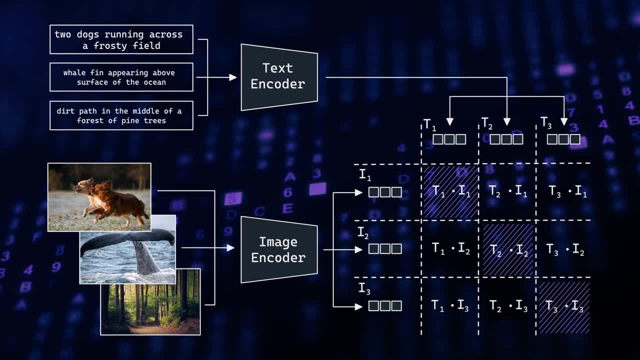 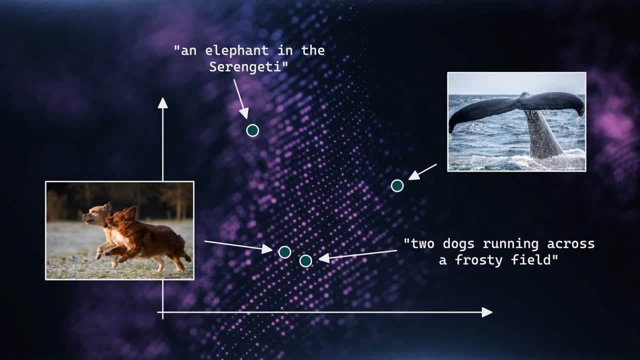 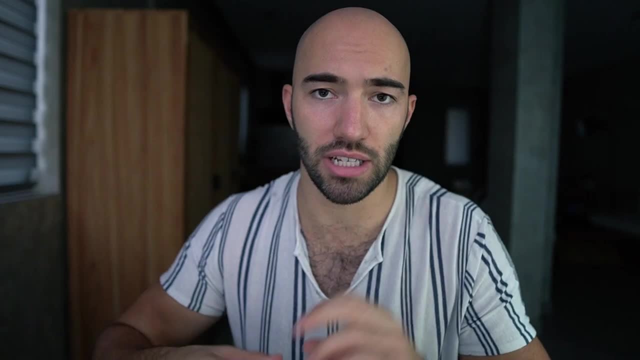 image encoding. Both of these models within CLIP are optimized during training in order to encode similar text and image pairs into the same vector space, whilst also separating dissimilar text and image pairs. so they are further away in vector space, So essentially in that vector space. 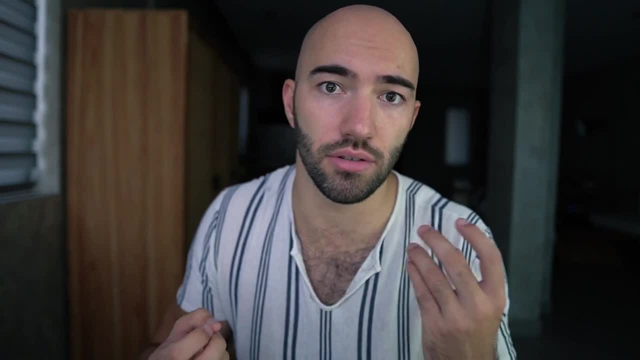 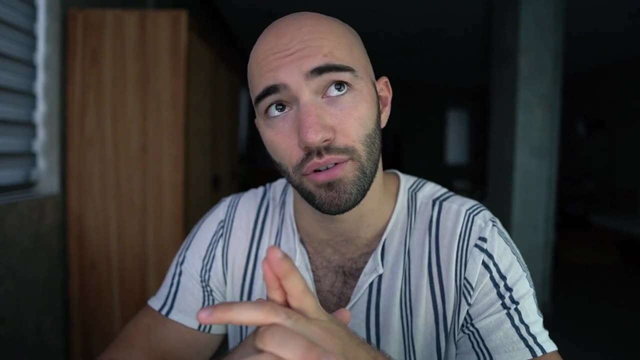 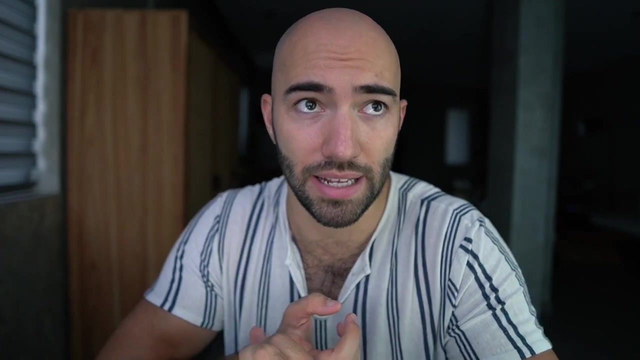 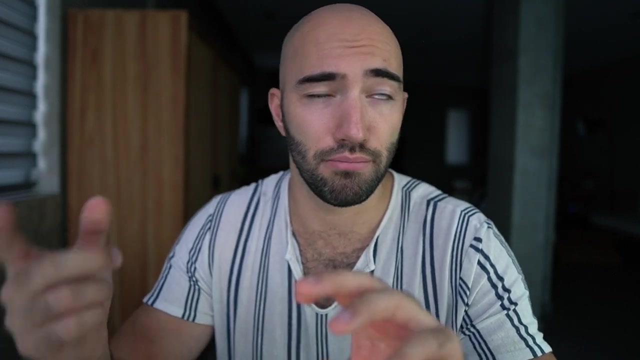 similar items are together. CLIP distinguishes itself from typical image classification models for a few reasons. First, it isn't trained for image classification and it was also trained on a very big data set of 400 million image to text pairs with this contrastive learning approach. So from this we get a few. 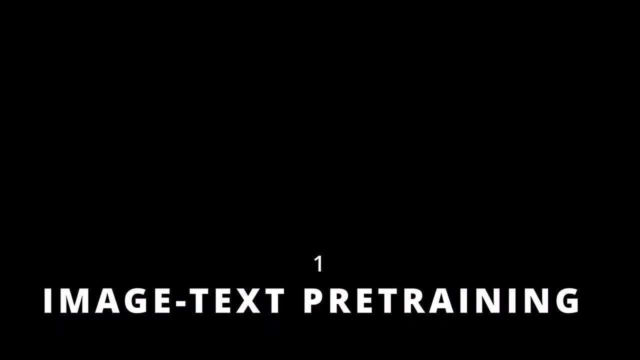 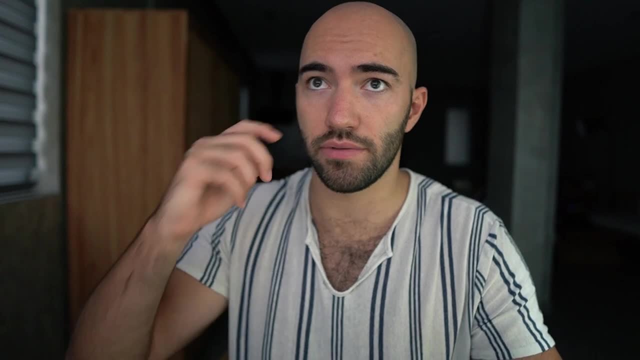 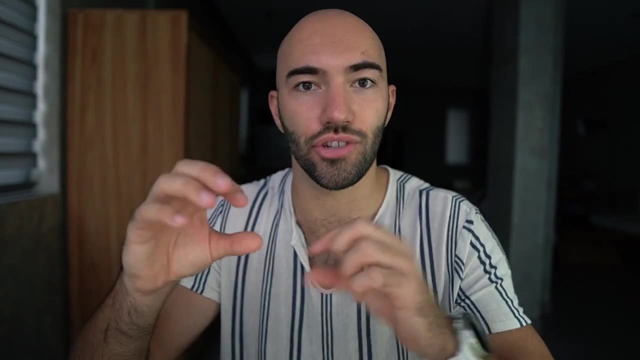 benefits. First, for actually pre-training the models. training the model, we can see that CLIP only requires image to text pairs, which in today's age of social media they're pretty easy to get. Any post on Instagram, for example, there's an image and there's usually a. 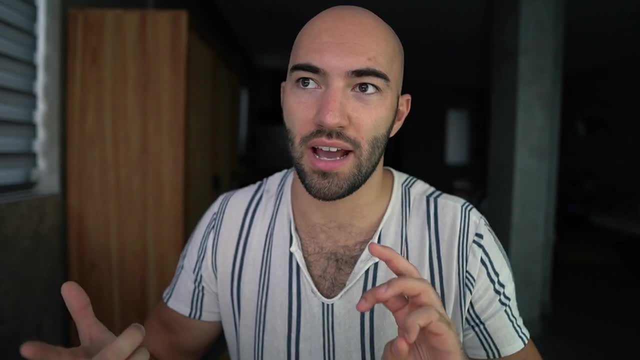 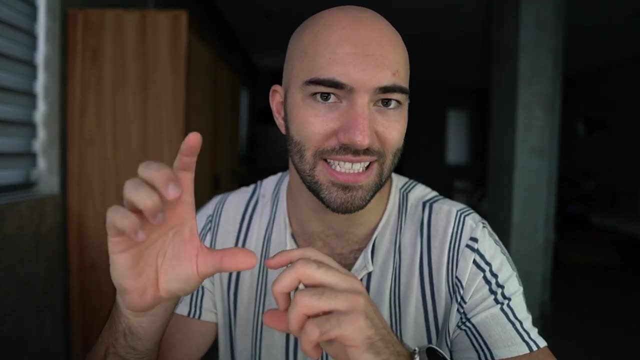 little caption of someone describing what is in the image. We have stock photo, websites, social media- you know just everything. everywhere We have images and text usually tied together, So there's a lot of data for us to to pull there Because of the large data set sizes that we can. 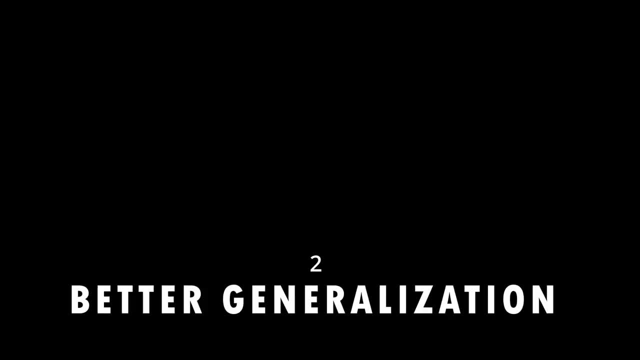 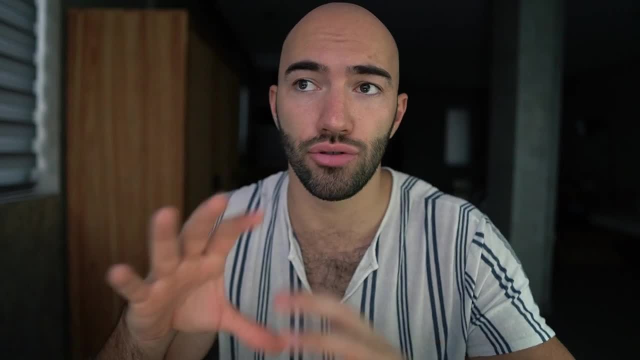 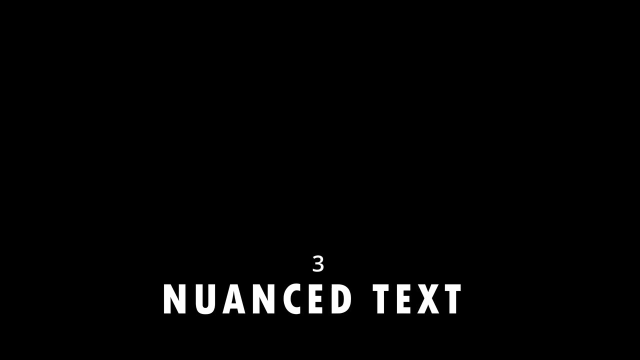 use with CLIP. CLIP is able to get a really good general understanding of the concepts between language and images and just a general understanding of the world through these two modalities As well. within these pairs, the text descriptions often describe the image, not not just one part of. 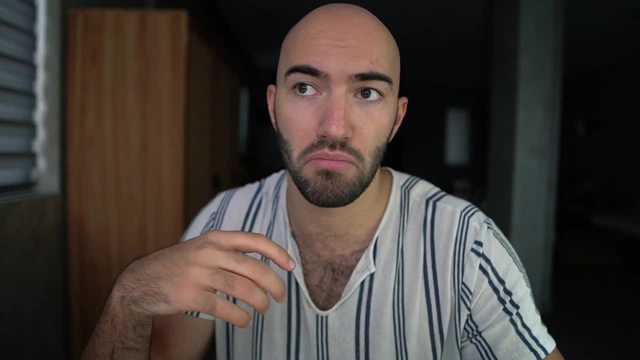 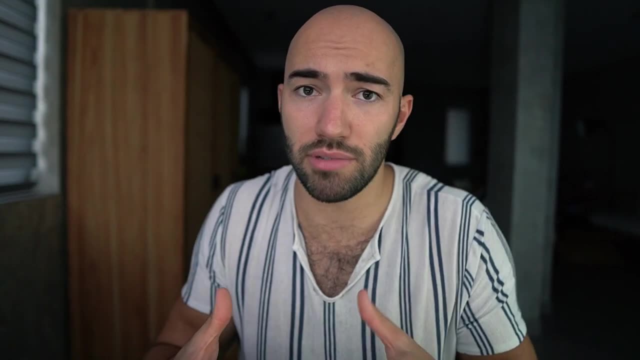 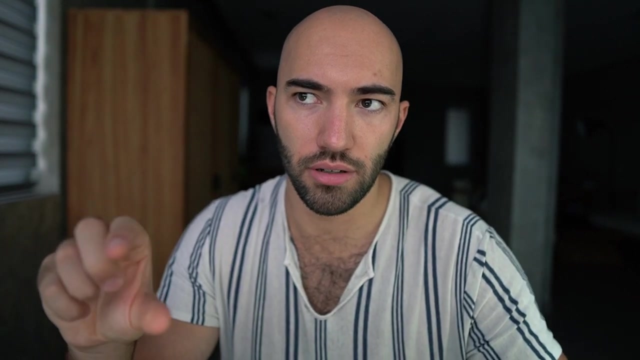 the image, like: okay, there's a dog in the image but something else, like a dog is running in a grassy field, okay, they describe something more and sometimes even describe very abstract things like the sort of feeling or mood of the photo. so you get a lot more information from these image text pairs than 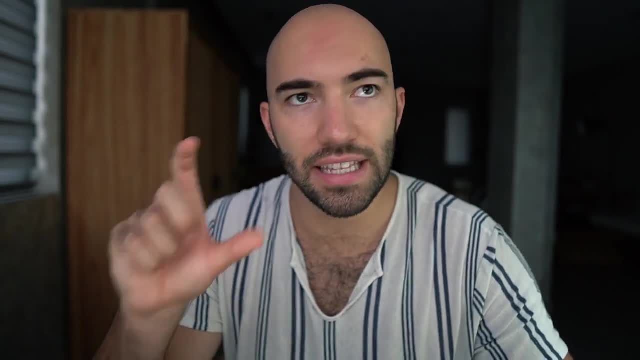 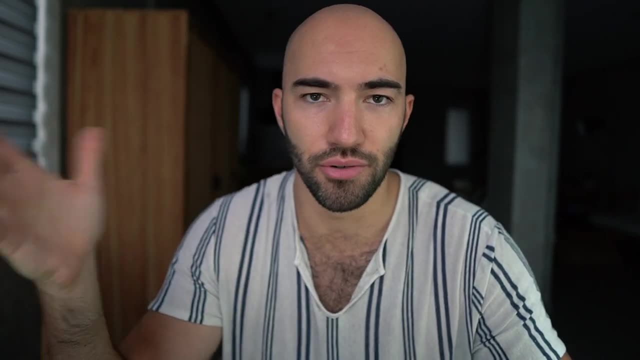 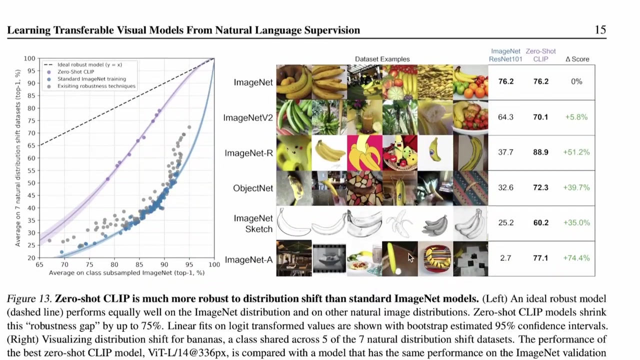 you do with a typical classification data set, and it's these three benefits of clip that have led to its pretty outstanding zero shot performance across a huge number of data sets. now the authors of clip. in the original clip paper they draw a really good example using clip and the resonet. 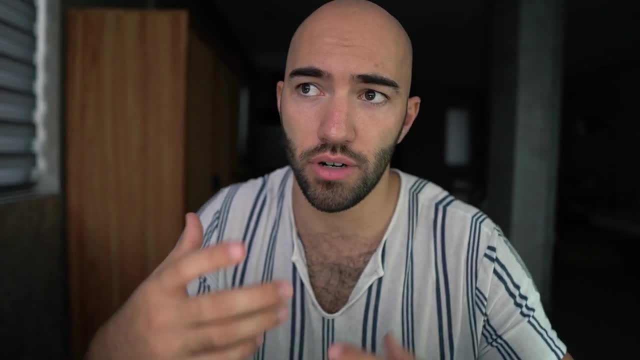 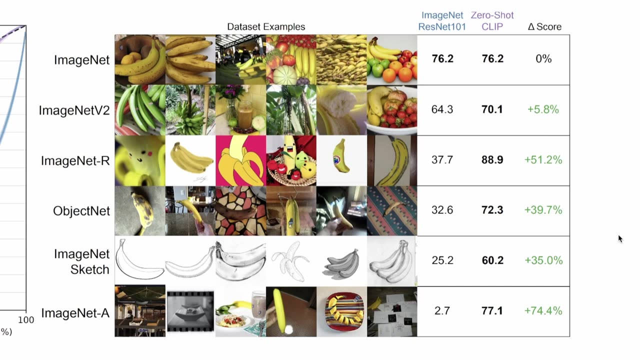 101 model trained for image net classification. now, clip was not trained specifically for image net classification, but they showed that zero shot performance with clip versus this state of the art model trained for image net was comparable on the actual image net data set. and then we learned that clip was not trained specifically for image net classification, but they showed 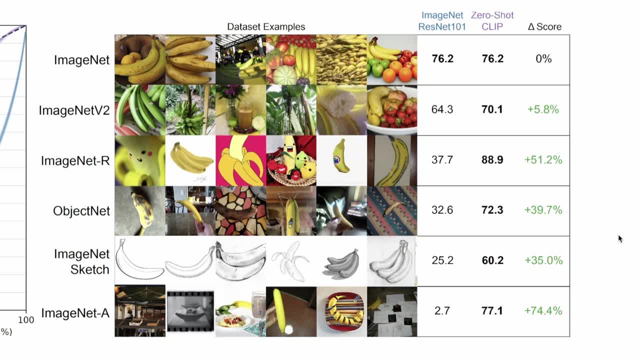 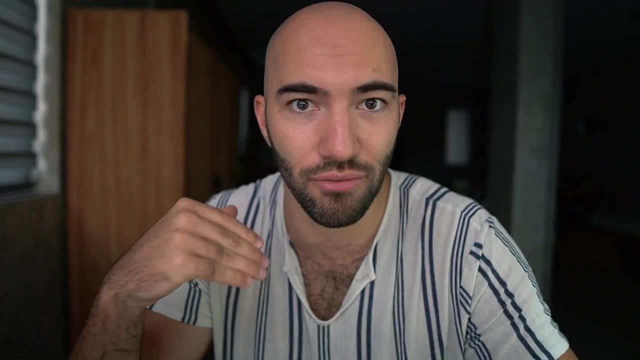 When we compare them on other datasets that are derived from ImageNet. so you have ImageNet V2, ImageNet R, Algenet, ImageNet Sketch and ImageNet A CLIP outperforms the model that was specifically trained for ImageNet on every single one of those datasets, which 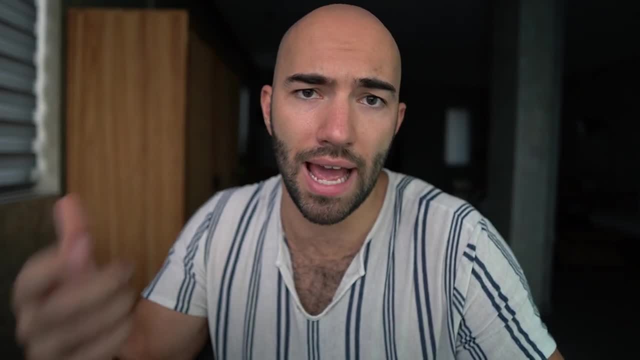 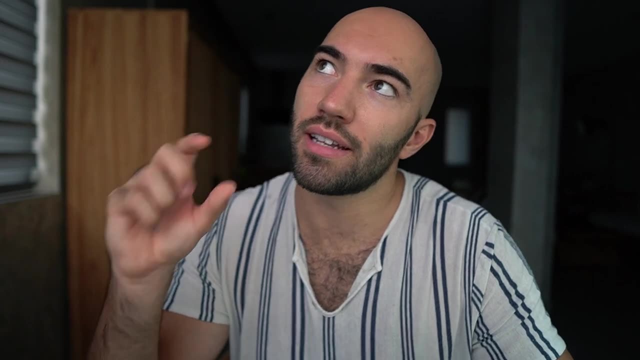 is really impressive. Okay, let's talk about how CLIP is actually doing zero-shot classification and how we can use it for that as well. So CLIP, or the two models within CLIP, they both output a 512-dimensional vector. 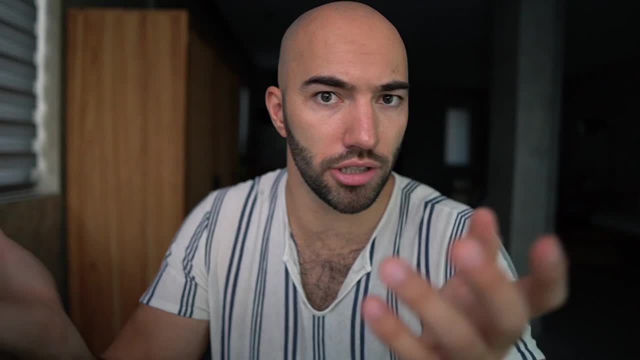 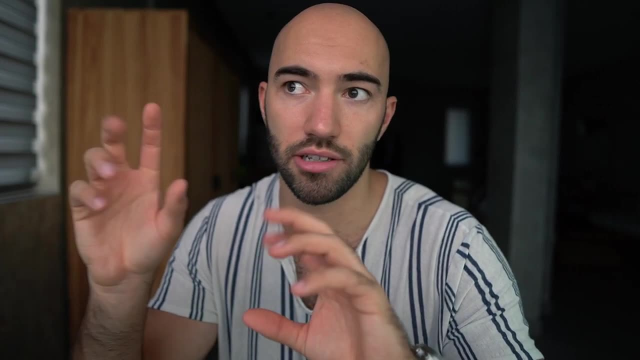 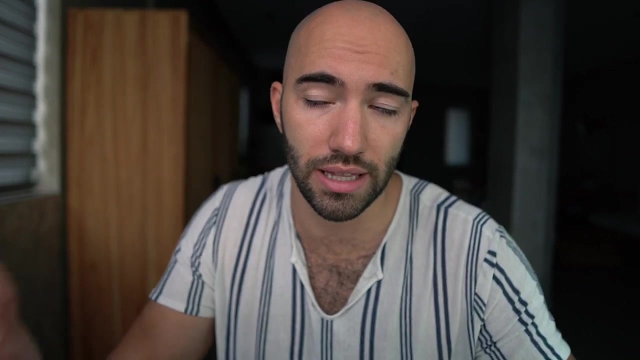 Now the text encoder. it can consume any piece of text, right, And then it will output a vector representation of that text within sort of CLIP vector space. Then if you compare that text to an image also encoded with CLIP, what you should find? 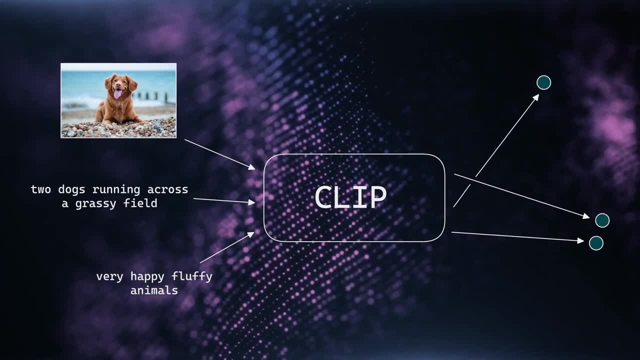 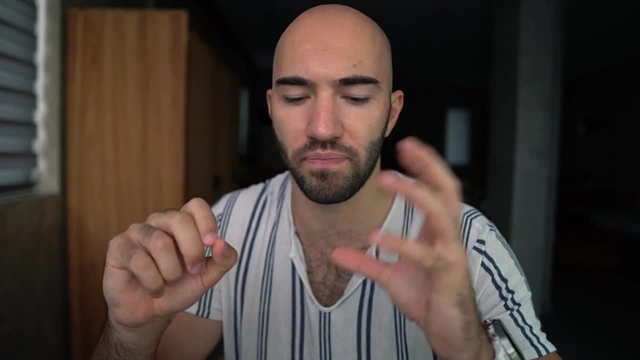 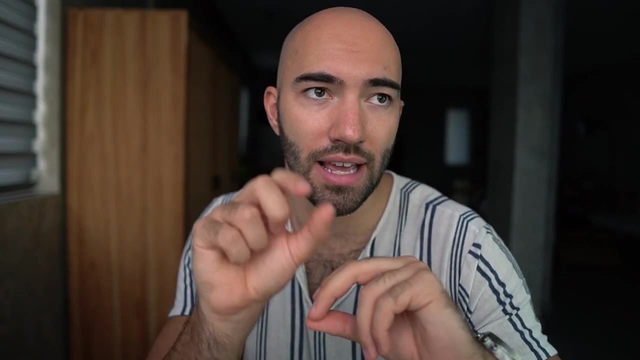 is that text and images that are more similar, Okay, Are closer together. So now imagine we do that, but instead of so we have our images from an image classification dataset and then for the text, we actually feed in the class labels for that classification. 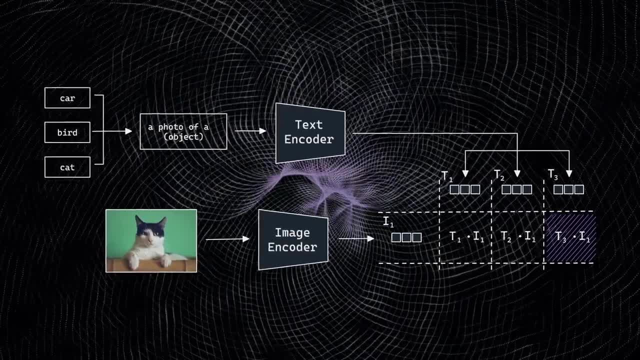 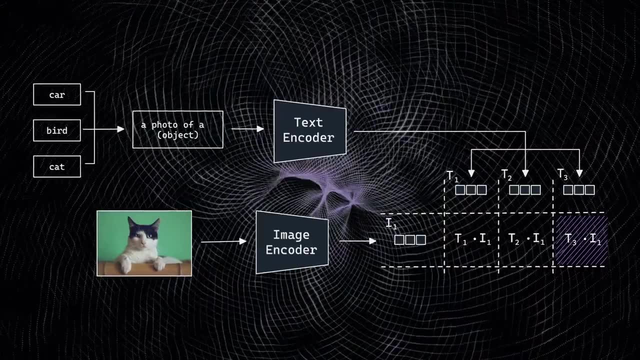 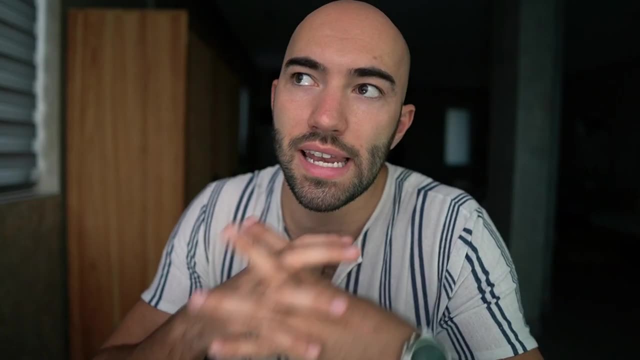 task. Then you process all that and then calculate similarity between the outputs and whichever of your text embeddings has a high similarity to each image. That is like your class okay, Your predicted class, Okay. So let's move on to an actual applied example and implementation of zero-shot learning with 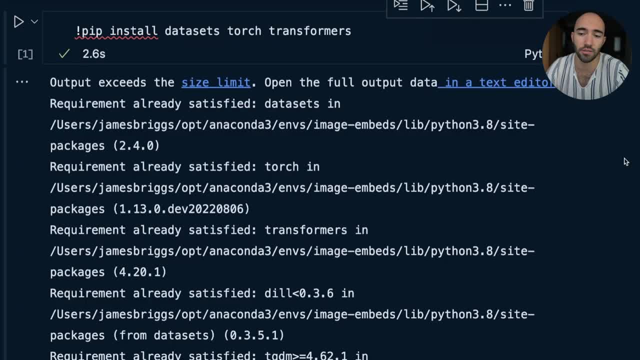 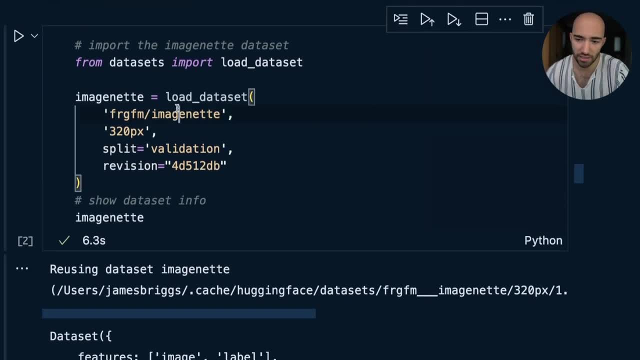 CLIP. Okay, So to start, we will need to pip, install datasets, Torch and Transformers, And what we're going to do is download a dataset. So this is the FRG FM ImageNet dataset. We've used this a couple of times before. 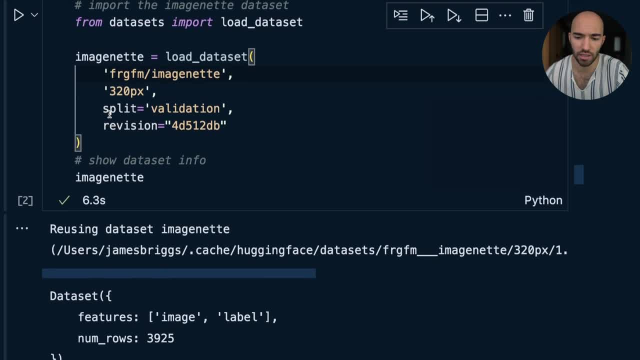 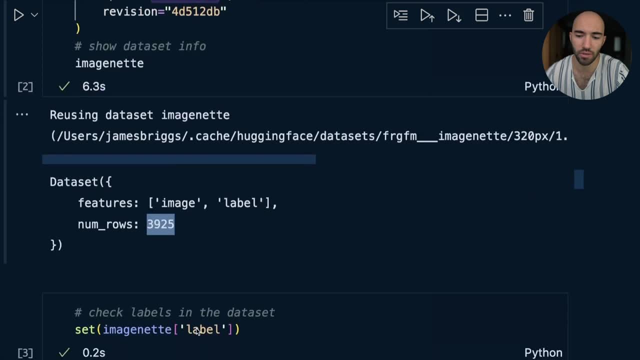 Okay, It just contains 10 different classes, not too much data here. we're looking at a validation set, So we have just under 4,000 items here. And if we have a look at what we have in the labels feature, so in the image feature, we 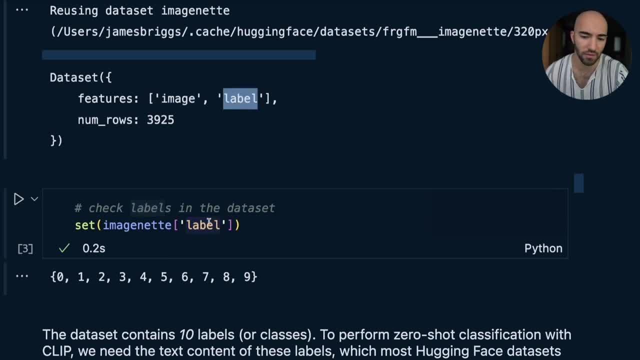 obviously have the images themselves label feature. We have these 10 labels- okay, But they're just numbers, they're integer values. We obviously need text for this to work with CLIP, So we need to modify these Or we need to map these to the actual text labels. 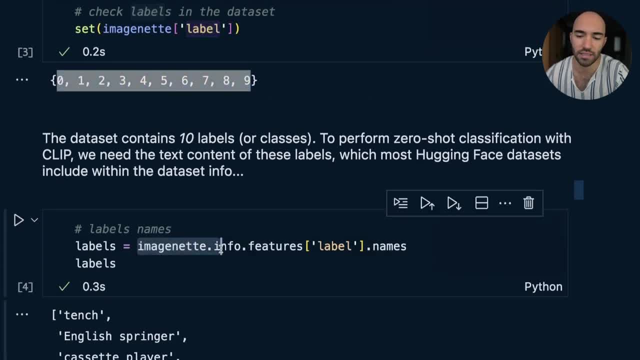 Now we do that by taking a look at the Hugging Face dataset info features and then label names. Okay, So most Hugging Face datasets will have a format similar to this, where you can find extra dataset information like the label names. 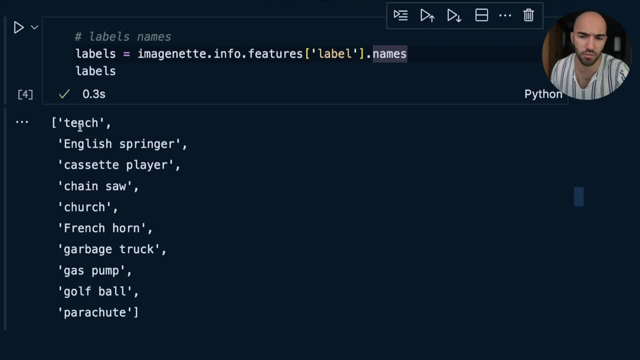 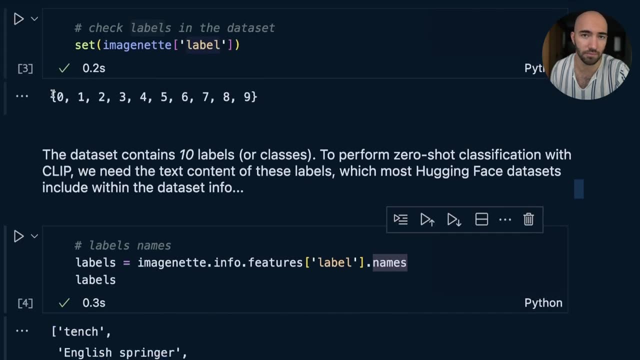 Okay, And then from there we can see we have 10, English Springer cassette player. you know a few different things. All of these map directly to the values here. So for zero we'd have 10, one would have English Springer, and so on. 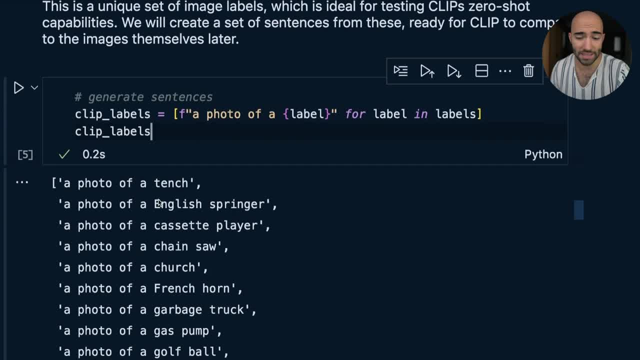 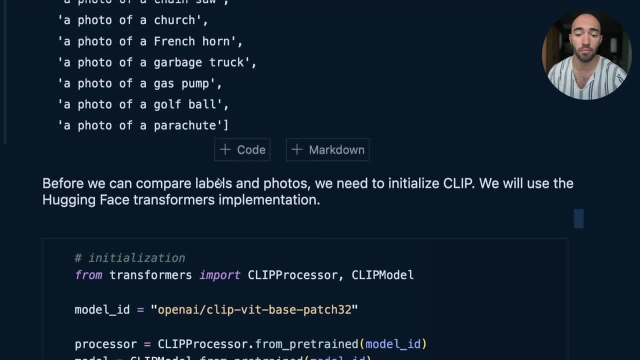 So, as before, we're going to convert these into sentences. So a photo of a 10, photo of a English Springer, and so on and so on. Okay, So from here, before we can compare the labels and the images we actually need CLIP. 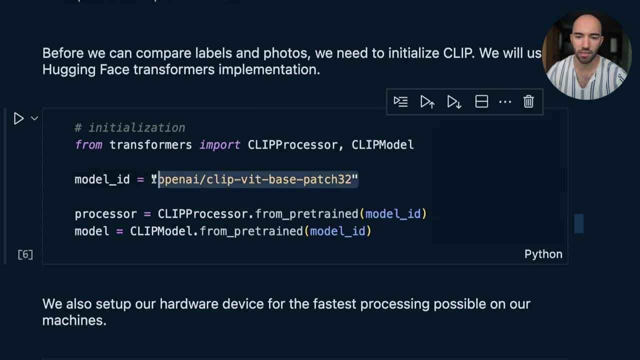 So we can initialize CLIP through Hugging Face. So we use this model here, Model ID, and then we use model processor which is going to pre-process our images and text, And then we also click model here, which is the actual model itself. 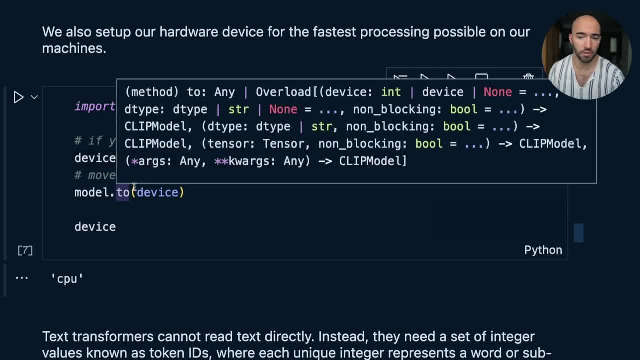 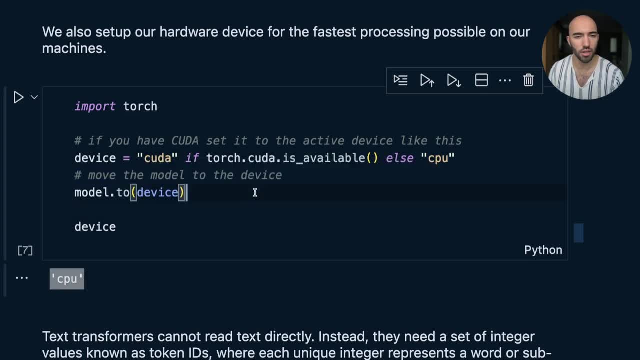 And then we can also run it on CUDA if you have a CUDA-enabled GPU. For me, I'm just running this on Mac, so CPU MPS, as far as I know, is not supported in full, or CLIP is not supported in full with. 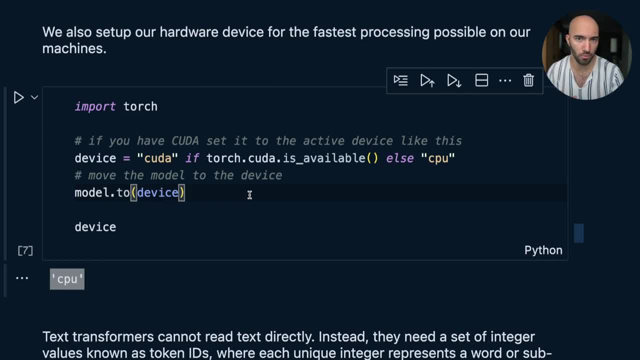 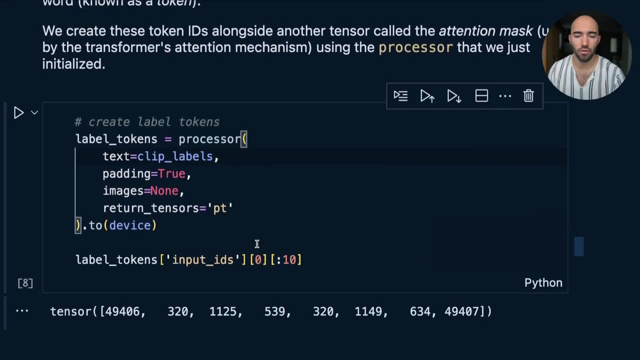 MPS yet, So that's like the Mac M1 version of CLIP. Okay, So that's the Mac version of CUDA For now. CPU is fast enough, it's not slow, so it's not a problem. Now, one thing here is that text transformers don't read text directly like we do. 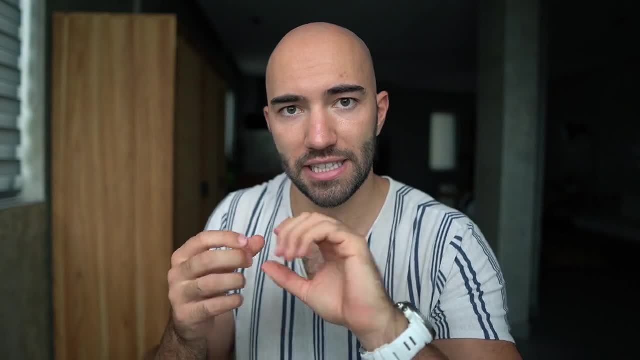 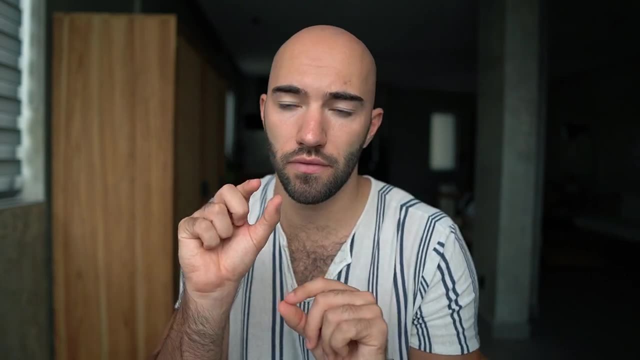 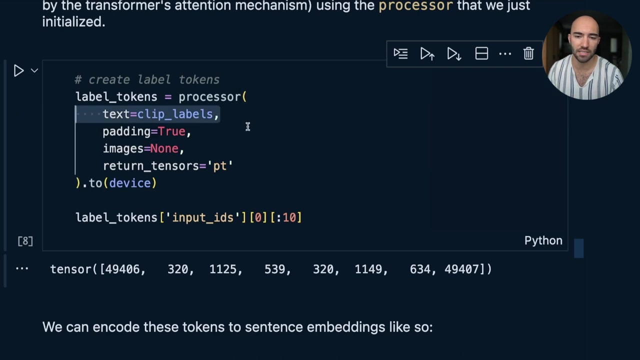 They need like a translation from text into what are called input IDs or token IDs, which are just integer representations of either words or sub-words from the original text. So we do that with the processor here. It's passing our text Padding we set to true so that everything is the same size. 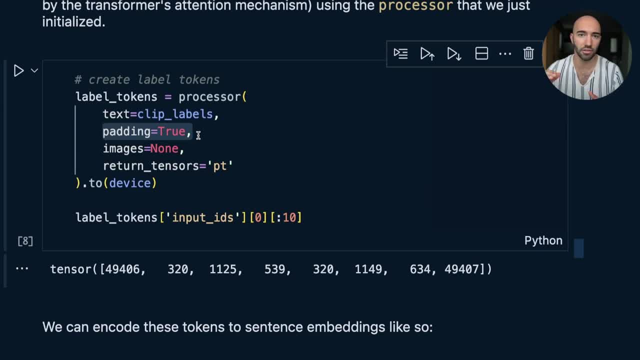 We need this when we're running things in parallel, multiple inputs in parallel, essentially when we're using batches. We're not passing our images here and we're going to return PyTorch tensors, Okay, And we're going to move all that to our device. 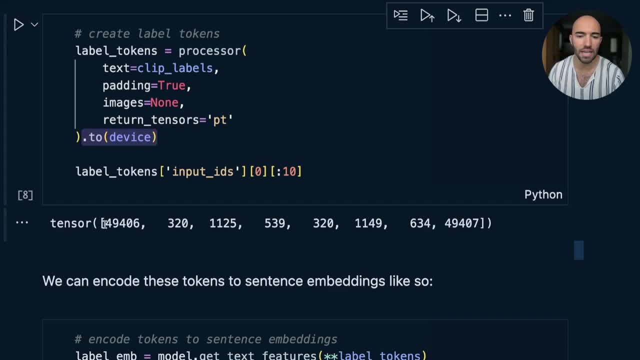 For me it's just CPU, so it doesn't actually matter, but it's fine. And then here we can see those tokens, So we have a starter sequence token here and then we could imagine: this is something like a photo, A photo of a tench. 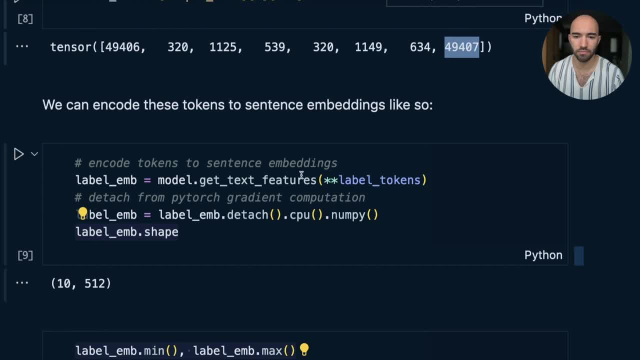 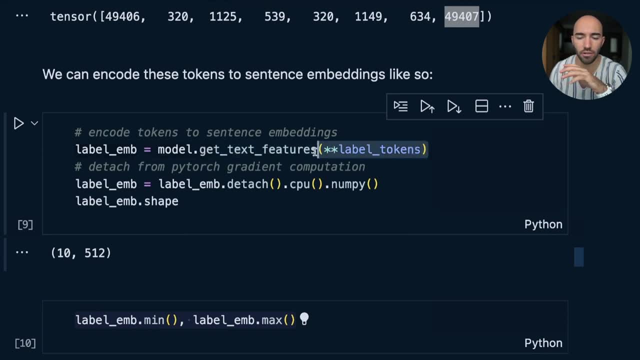 Something along those lines, And then end of sequence over there as well. So we can encode these tokens into sentence embeddings. All we do is this: So pass our sentence. sorry, our tokens in here: label tokens. Now, in here we have input IDs and also another tensor called attention mask. 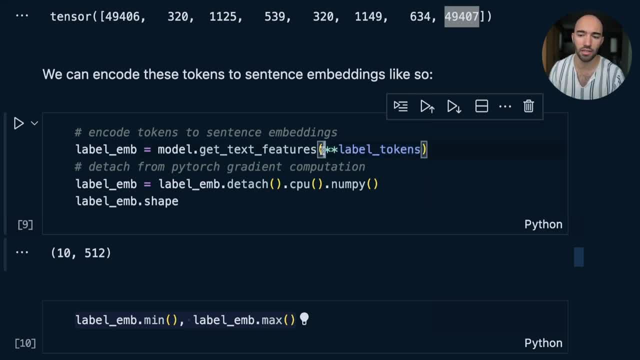 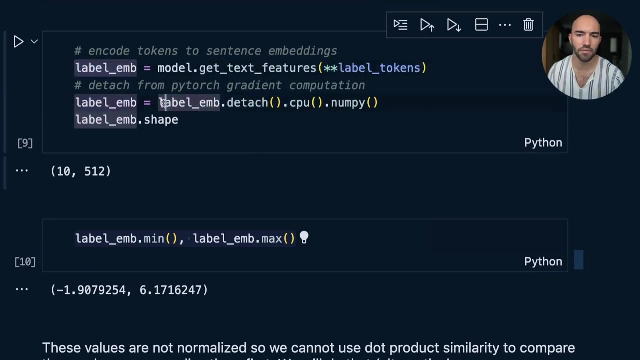 And that's kind of wrapped within a dictionary, which is why we're using these two asterisks here to iteratively pass both of those tensors. So we could also pass individual items to the get text features function And then, after we have our label embeddings over here, we sort of detach them from PyTorch. 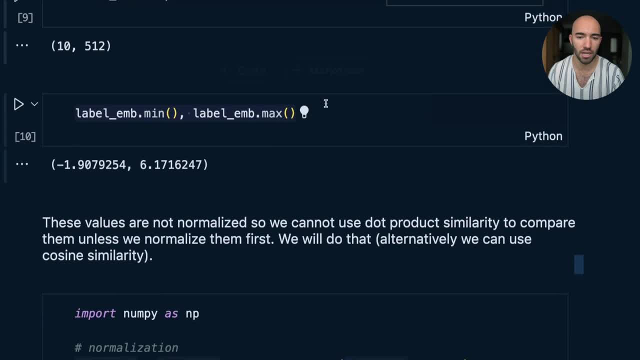 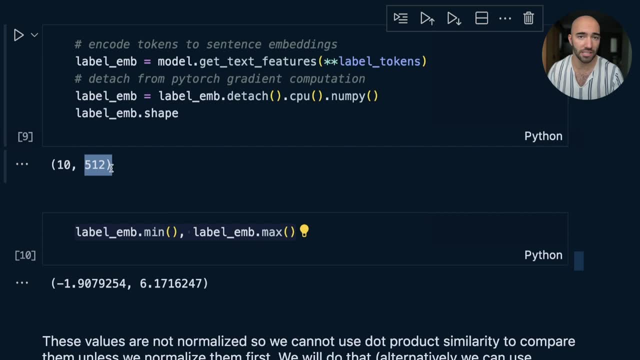 gradient computation of the model and convert that into numpy, And then we can see from that that we get 10 512 dimensional embeddings. Okay, So they're now the text embeddings within that click vector space, And one thing to note here is that they're not normalized. 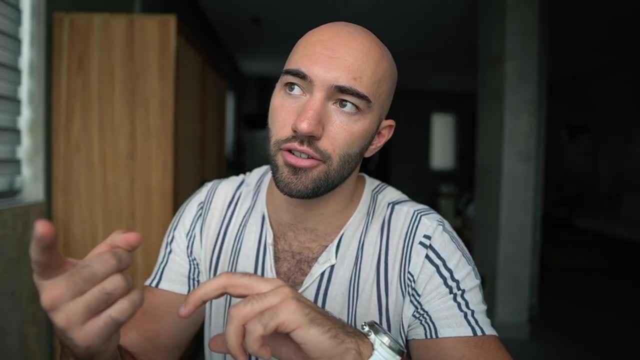 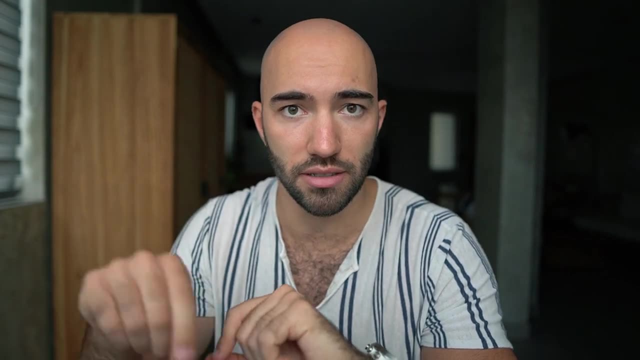 Okay, can see they're not normalized. so we can either use cosine similarity to compare them, or we can normalize them and then we can use dot product similarity. now, if we normalize first, I find the code later on to be simpler, so we will do that here. 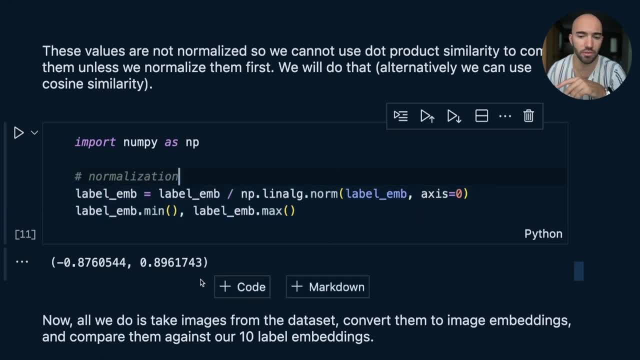 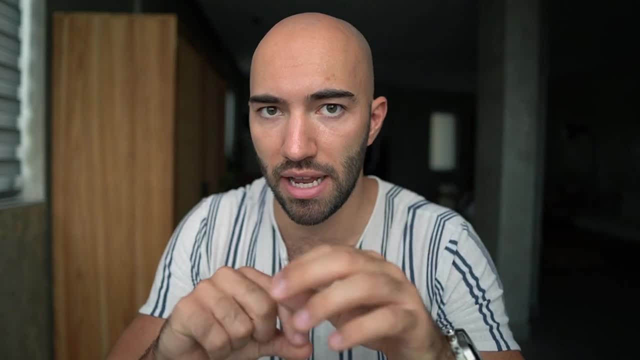 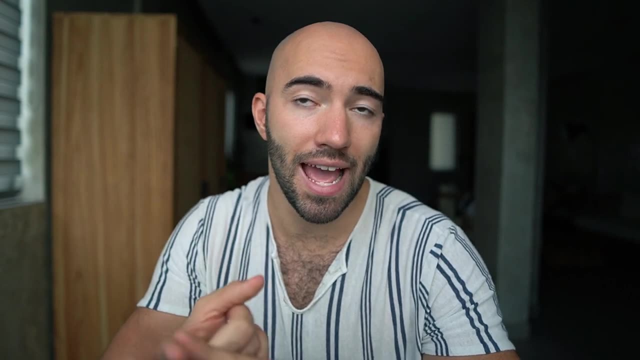 so we're going to normalize here. it's pretty simple and then we can see straight away they're normalized. we can just use dot product similarity. now that's the text embedding or the label embedding part. now what we want to do is have a look at how we do the image embeddings and then how we compare them. 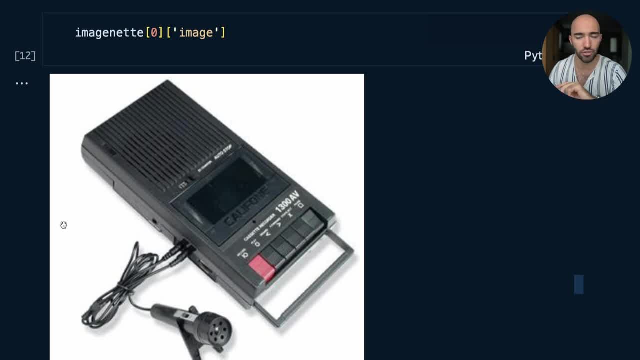 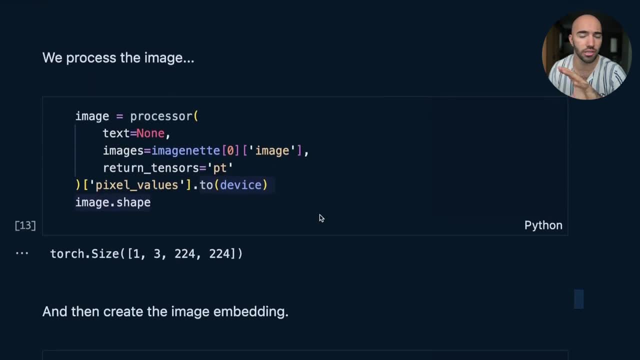 so we're going to start with this image first, just a single image. we'll go through the whole dataset in full later. so we just have a cassette recorder here. now we go down here, we're just going to process the image. so, using the same processor, we set text to none, because no text this time and what we want to do is: 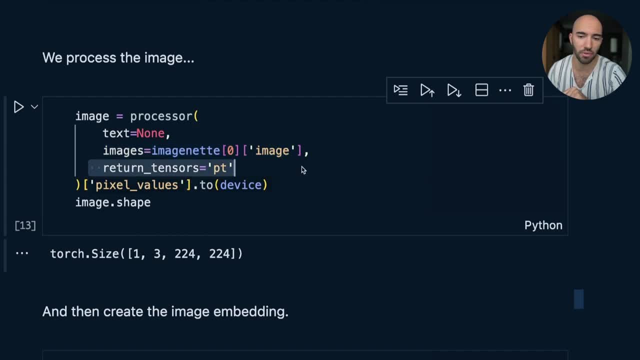 just pass that image in here to images and we're going to return the tensors- it's PyTorch tensors- and extract the pixel values. now the reason that we have to process the image is clip expects every tense that it sees to be normalized, which is the first thing it does, and also a particular shape. it. 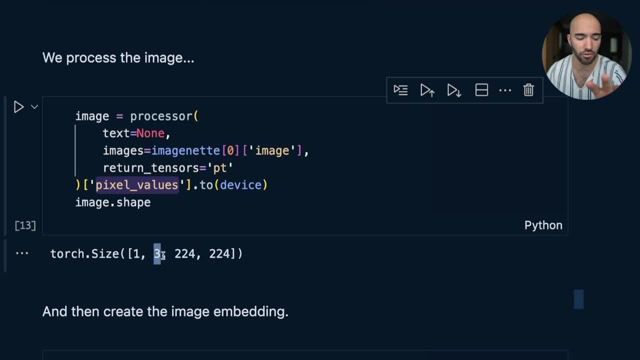 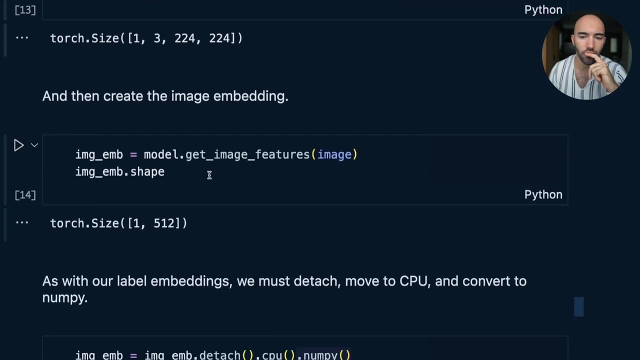 expects this shape here. so three color channels, which is through here, a 224 pixel wide image and 224 pixel height image. okay, so all we're doing there normalization and resizing, and then from there we can pass it to get image features. image again like here: we didn't, we didn't. 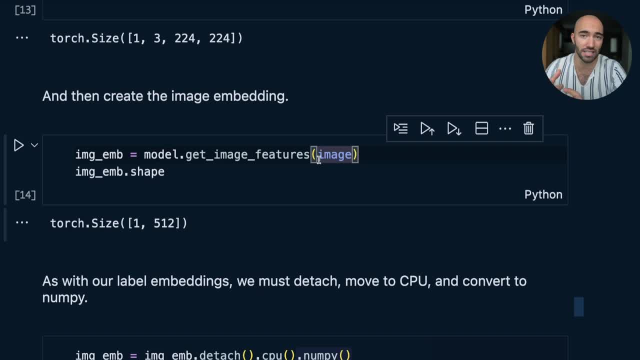 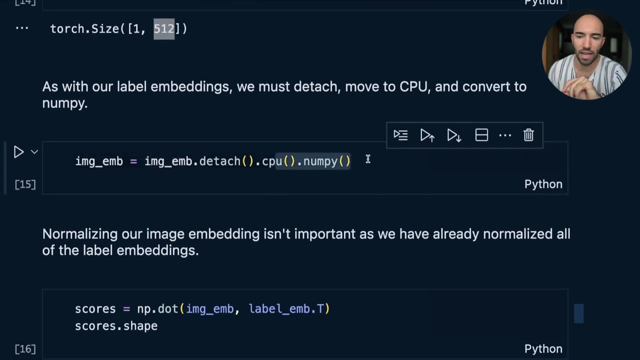 include the iterable, because this is just a single tensor. we don't need to pass the two asterisks here and we get a single embedding here, one vector which is 512 dimensions. as with our label embeddings, we're going to detach them, move them to CPU and then convert to numpy. I already have them on CPU, so this: 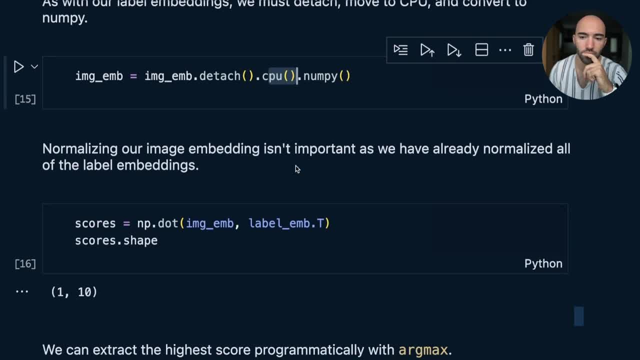 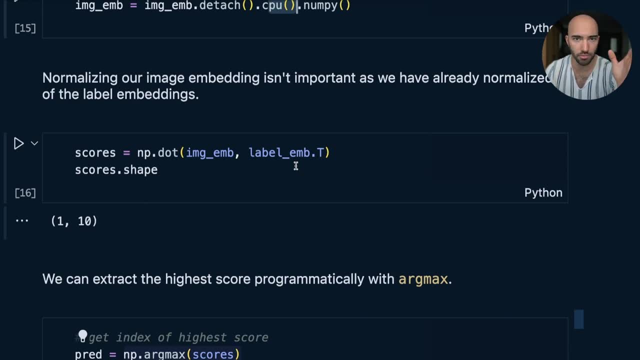 part isn't necessary, but if you're using CUDA it will be, and then we don't need to normalize them. so when we're doing dot product similarity, we just need one side of the calculation to be normalized, not both. okay, so with that we do numpy dot, we have our image embedding and then we 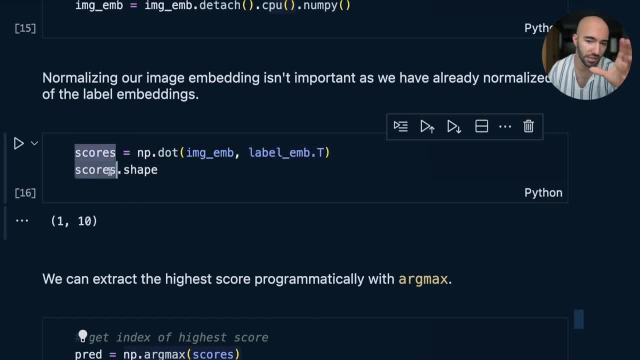 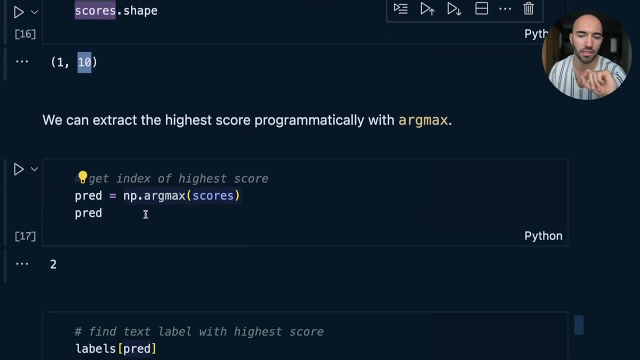 transpose label embeddings and you see that we get scores, and the shape of those scores is one dimension that's not important here. we have those 10 similarity scores, so one similarity value for each of the our 10 labels. okay, so then we can take the index of the highest score, which? 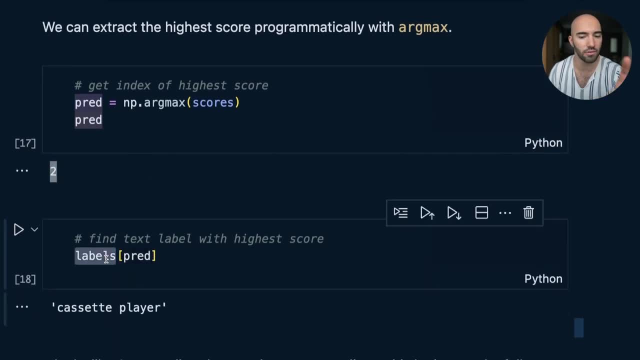 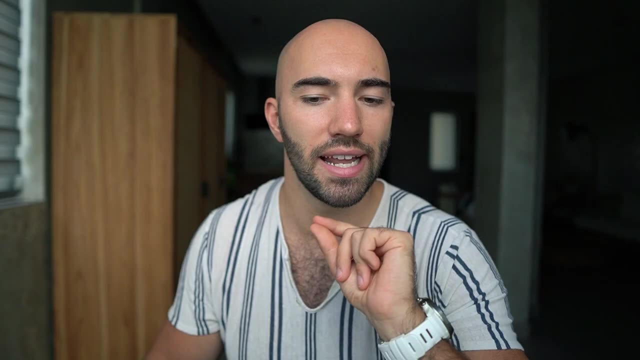 happens to be index 2, and then we find out, okay, which which label is, that it is cassette player. okay, so it's correct. that's pretty cool. now let's have a look how we do that for the whole data set. so all I'm going to do is we're going to go. 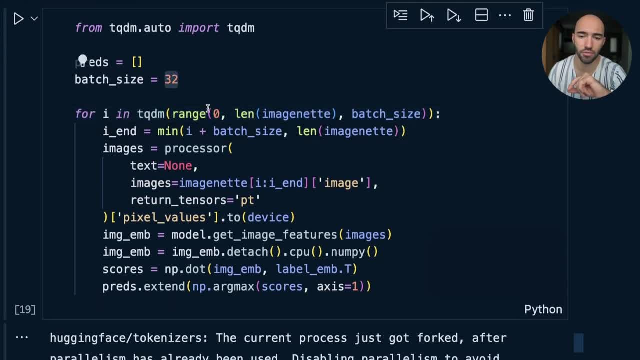 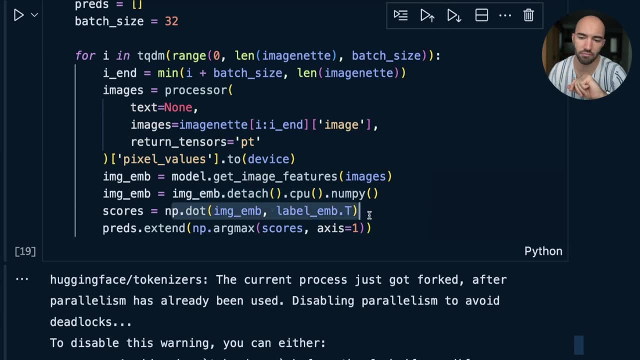 through in a loop, through the whole data set. we're going to do it in batches of 32: process everything. this is all just the same stuff: process, get the embeddings, get dot product. okay, we don't need to redo this for the labels, because we we just have the 10 labels throughout the whole thing. 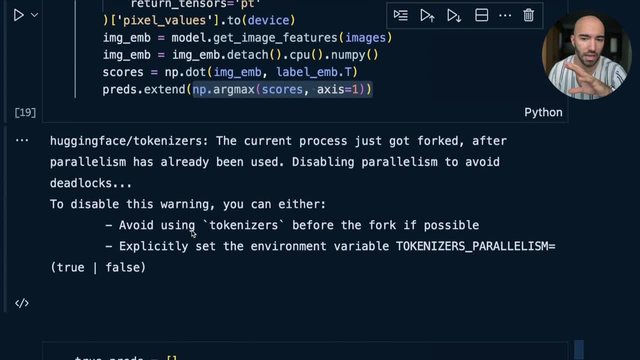 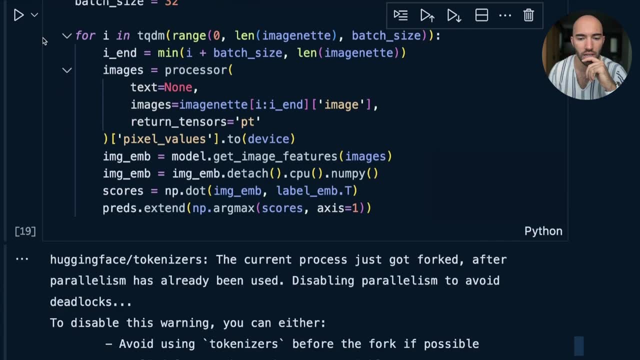 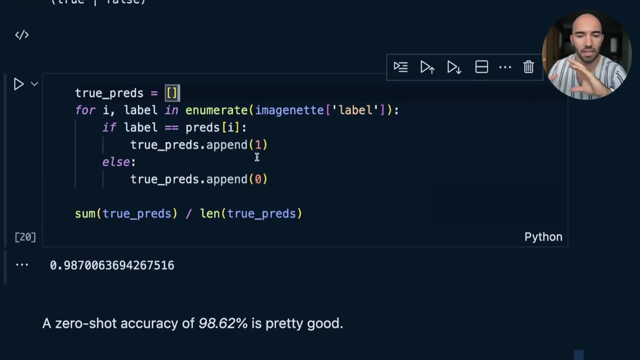 so it's not necessary. we'll get the argmax and we're just gonna append or extend a prediction list with all of those predictions, okay, and let's see what we get. well, let's see what the performance is there. so here, calculating how many of them align to the true values. 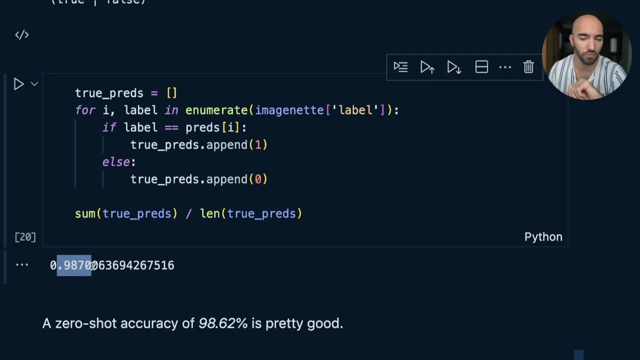 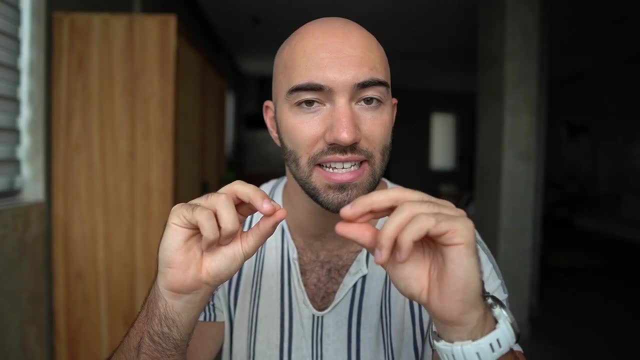 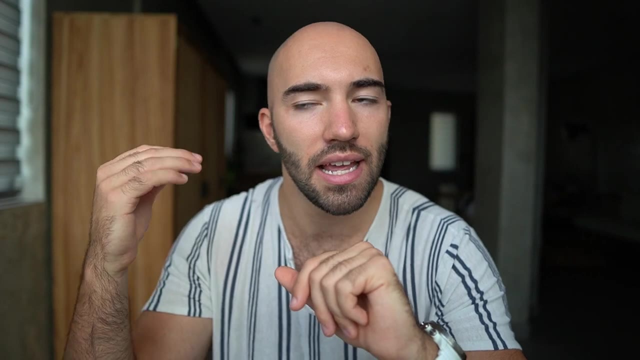 and we can see you get 0.987 okay. so that means we get 98.7 percent accuracy, which is pretty insane when you consider that we have done no training for clip here. it has not seen any of these labels. it has not seen any of these images. this 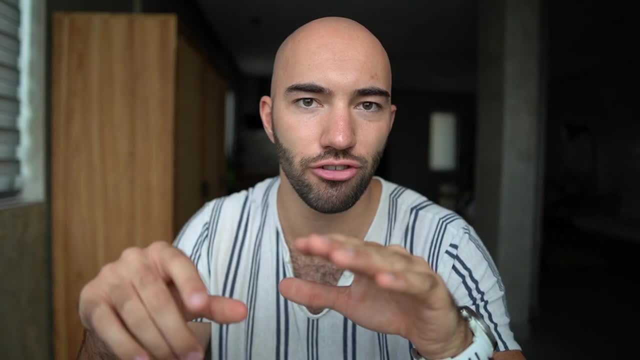 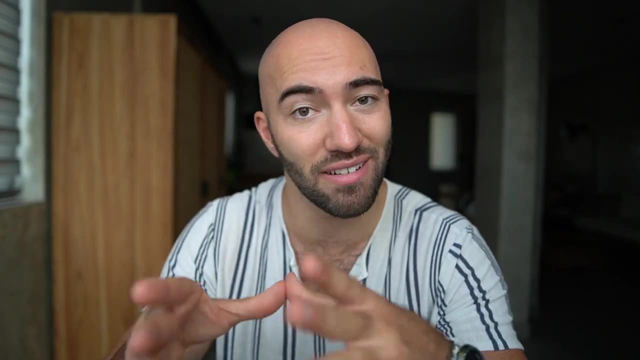 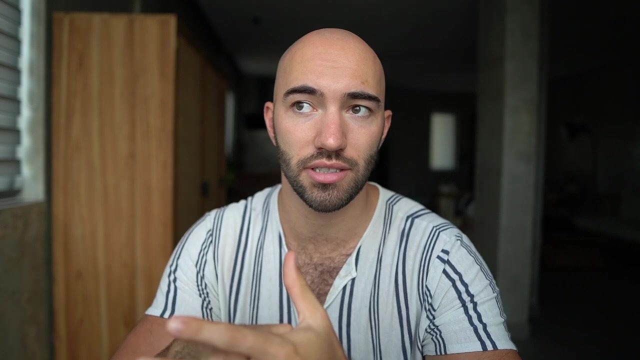 is my out-of-the-box zero-shot classification and it's scoring 98.7 percent accuracy, which is, I think, really very, very impressive. so this is, uh, i think, a good example why i think zero shot classification, or image classification with clip, is such an interesting use case. um, it's just so easy. 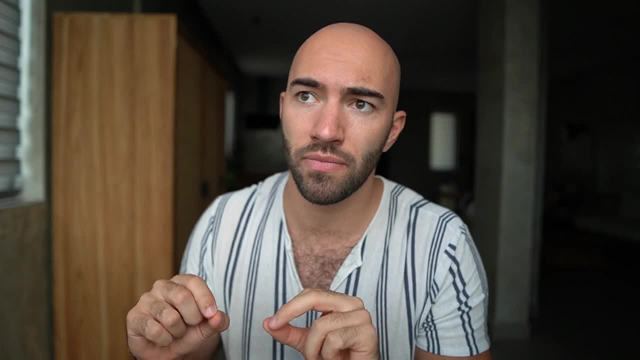 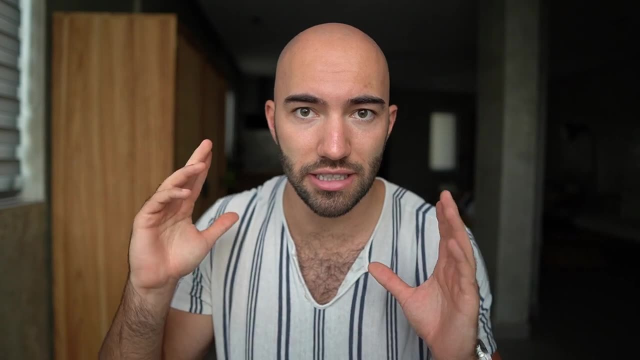 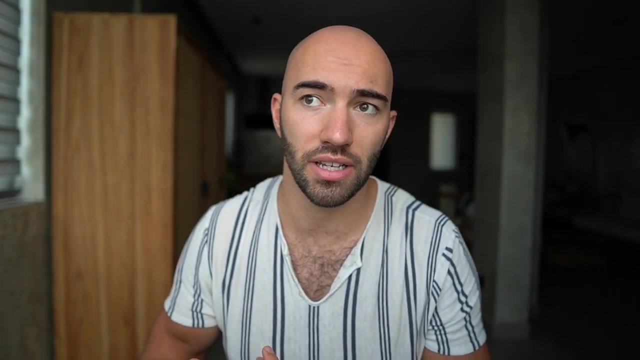 right, you can do this for a whole ton of data sets and get good performance. it's not going to be state-of-the-art performance, but pretty good performance, like like this, super, super easy. so before clip i, as far as i'm aware, this sort of thing was impossible. okay, every, every domain. 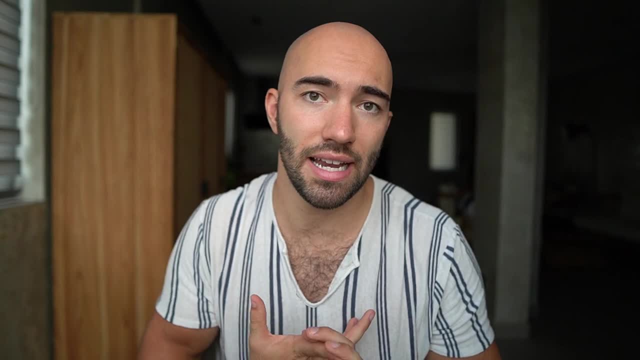 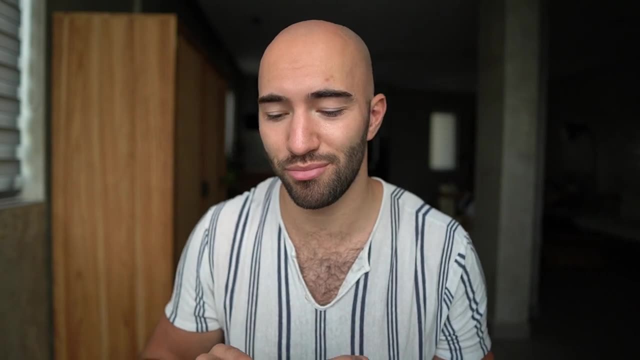 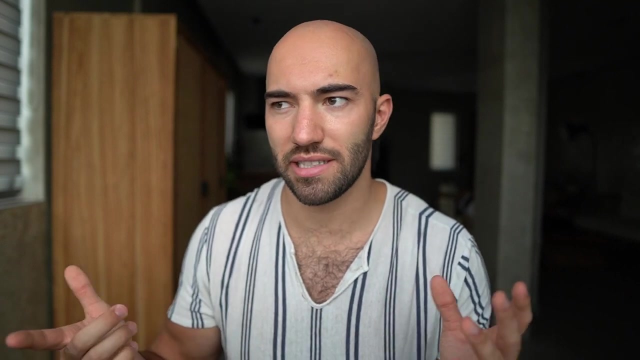 adaption to a new classification task needed training data, it needed training, and so on. with this, it's just a case of you need to write some labels, maybe modify them into sentences, and then you're- you're good to go. so that's why i think clip is. i think it has created a pretty